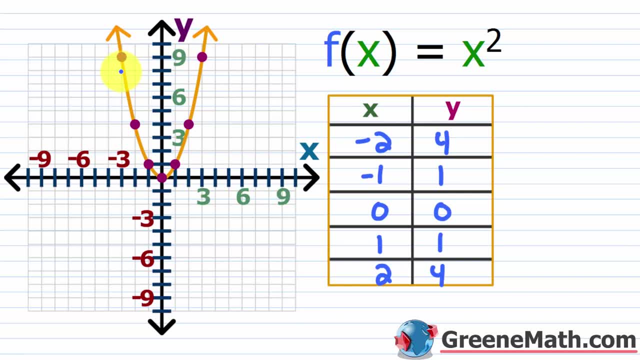 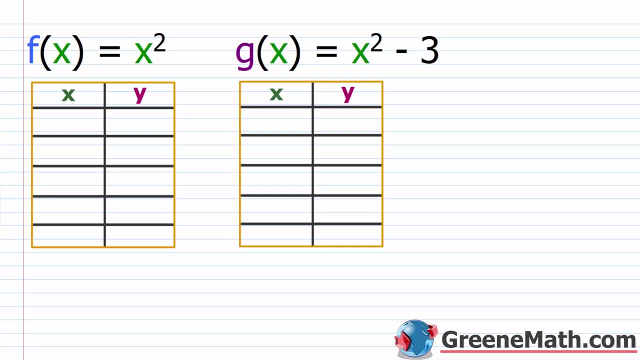 4,16 as well. All right, let's look at the next kind of part, and what we're going to do now is just kind of compare tables. We're going to look at this other function that's very close to the original. So we have f of x equals x squared. 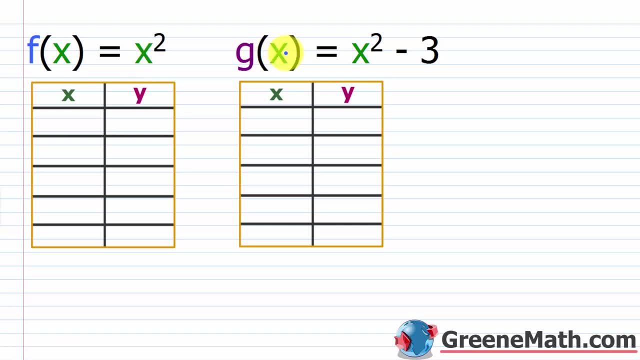 We're going to call this the parent function, okay. And then g of x is going to be kind of this guy, but just a little bit different, okay, So g of x is x squared minus 3.. So this part right here and this part, those are the same. right, You have that x squared. but 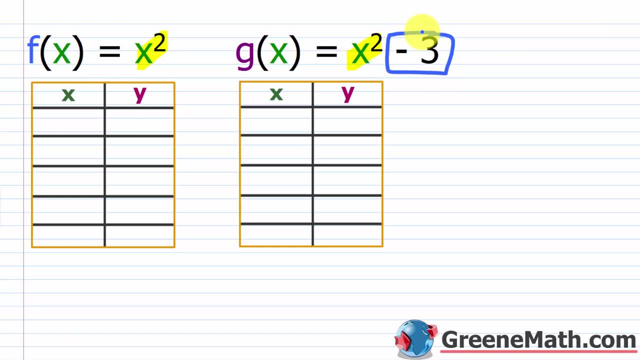 now you have this extra minus 3. that's involved, okay, And the way your book is going to show this to you, they're going to say that g of x can be defined as f of x, which is just x squared, so f of x and then minus this 3, okay. 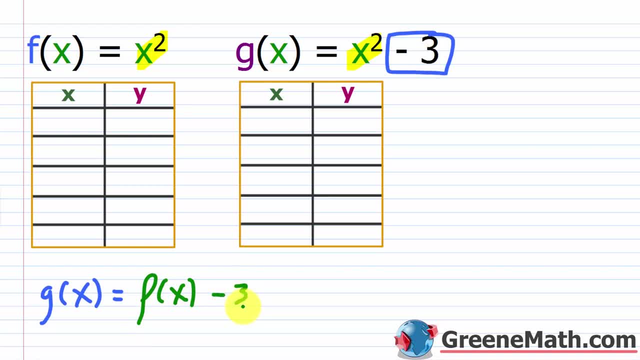 So minus this 3.. So let's look at these kind of two tables real quick and I'll show you what's really going on here. So again, we know these by heart. So, negative: 2, 4, negative: 1, 1, 0, 0, 1, 1, and 2, 4, okay, But what's going to happen over here? We know that we. 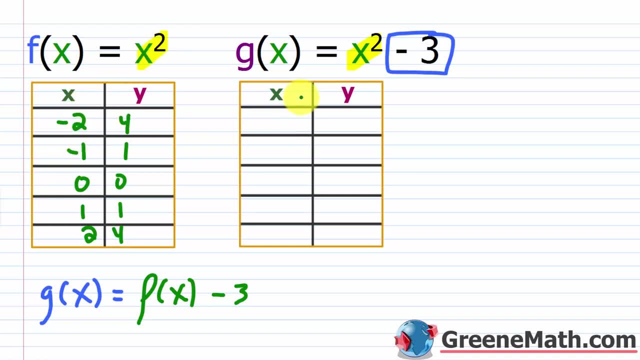 got these values by plugging in something for x and squaring it. But over here I plug something in for x and I square it, but then I subtract away 3, okay. So whatever, I got over here for y, okay for a given x value. now over here for y, it's going to be 3 less. 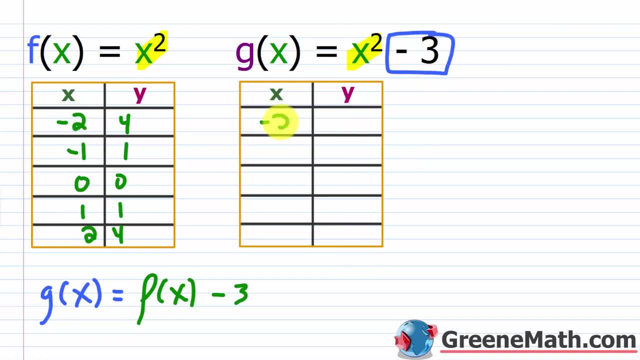 of this minus 3.. So if I copy these same x values- so negative 2, negative 1,, 0,, 1, and 2, the y values associated will now just be 3 units less right. So instead of 4, it. 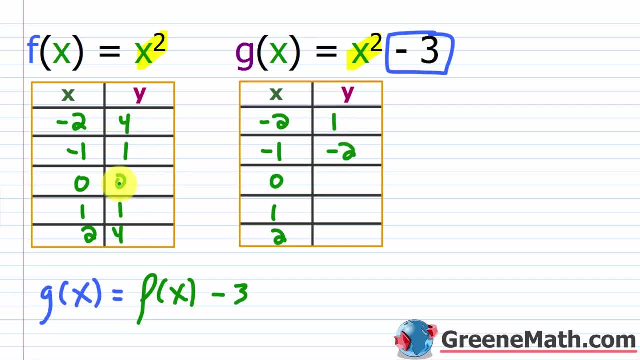 would be 1.. Instead of 1,, it would be negative 2.. Instead of 0,, it would be negative 3.. And then, instead of 1,, again it would be negative 2.. And again, instead of 4, it would be 1.. 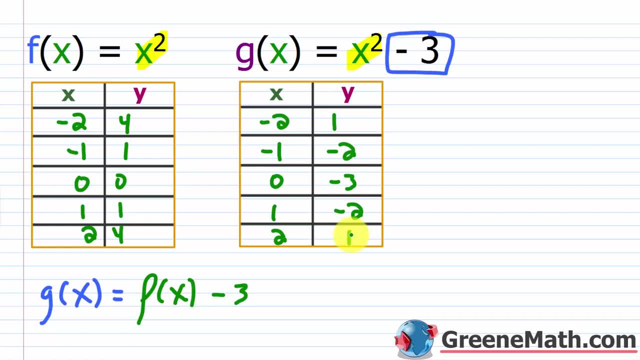 Now what effect do you think this will have graphically? Think about this real quick: A given x value. now the y values have been decreased by 3 units. Remember the y axis is a vertical axis. So what's going to happen is this is going to shift the graph down. 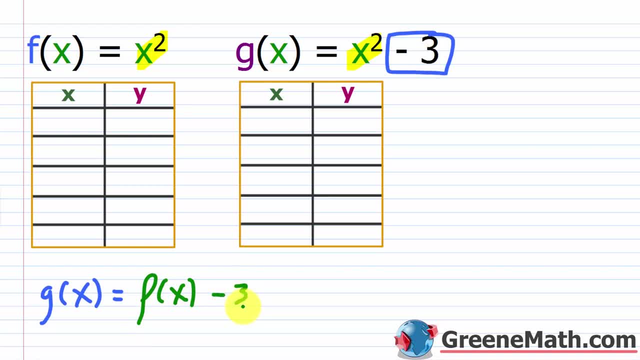 So minus this 3.. So let's look at these kind of two tables real quick and I'll show you what's really going on here. So again, we know these by heart. So, negative: 2, 4, negative: 1, 1, 0, 0, 1, 1, and 2, 4, okay, But what's going to happen over here? We know that we. 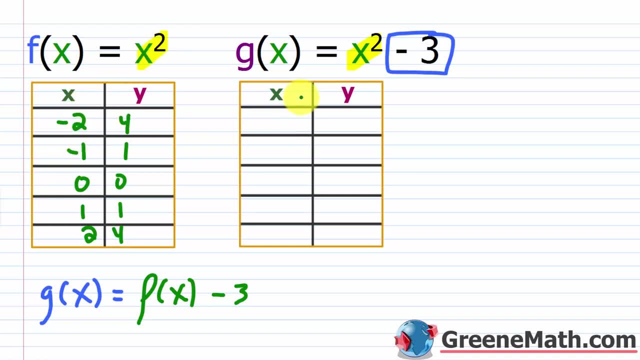 got these values by plugging in something for x and squaring it. But over here I plug something in for x and I square it, but then I subtract away 3, okay. So whatever, I got over here for y, okay for a given x value. now over here for y, it's going to be 3 less. 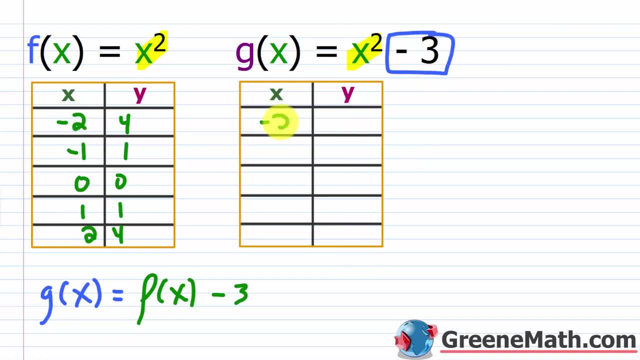 of this minus 3.. So if I copy these same x values- so negative 2, negative 1,, 0,, 1, and 2, the y values associated will now just be 3 units less right. So instead of 4, it. 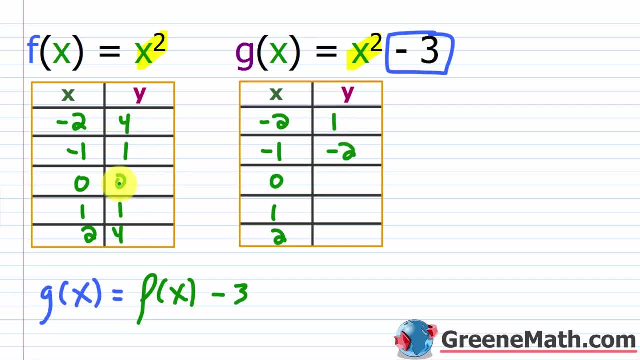 would be 1.. Instead of 1,, it would be negative 2.. Instead of 0,, it would be negative 3.. And then, instead of 1,, again it would be negative 2.. And again, instead of 4, it would be 1.. 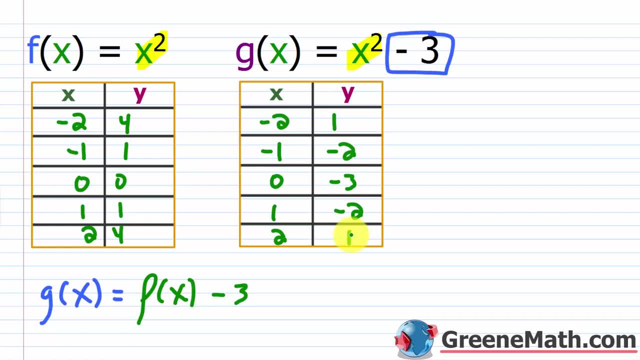 Now what effect do you think this will have graphically? Think about this real quick: A given x value. now the y values have been decreased by 3 units. Remember the y axis is a vertical axis. So what's going to happen is this is going to shift the graph down. 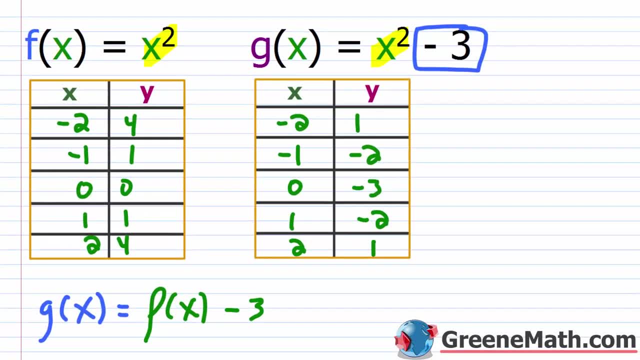 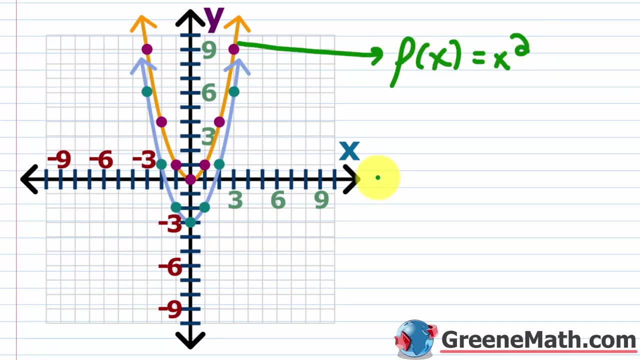 okay, by 3 units. Let's take a look at that real quick. So the orange graph is my original f of x is equal to x squared, And the graph in light blue- okay, the graph in light blue is my g of x is equal to x squared minus 3.. 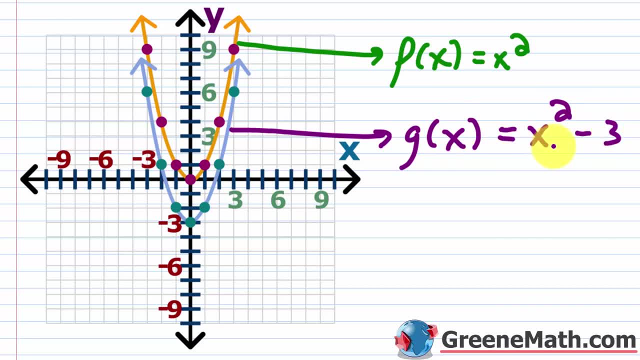 Okay. so if you wanted to graph g of x, if you got this on a test and they said: hey, graph x squared minus 3, you know that you just need to graph x squared and then just shift it down by 3 units. The easiest way to kind of do this is just to pick these points. 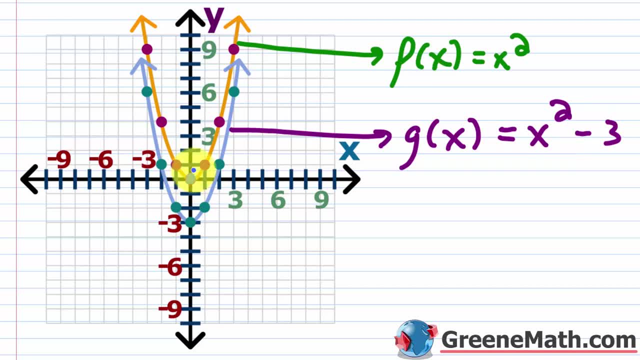 that you already know something like: let's say 0, 0, and say, okay, now it's going to be at 0, negative 3.. So that's my lowest point there, And then other points are just going. 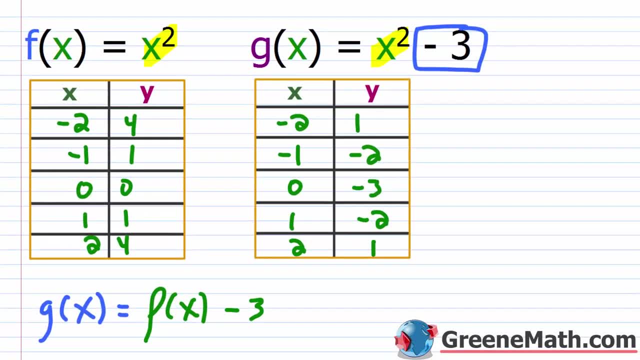 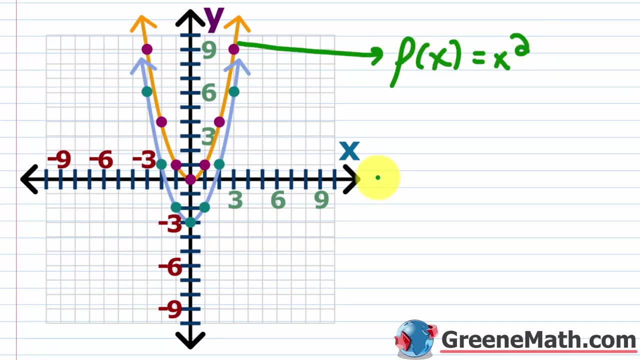 okay, by 3 units. Let's take a look at that real quick. So the orange graph is my original f of x is equal to x squared, And the graph in light blue- okay, the graph in light blue is my g of x is equal to x squared minus 3.. 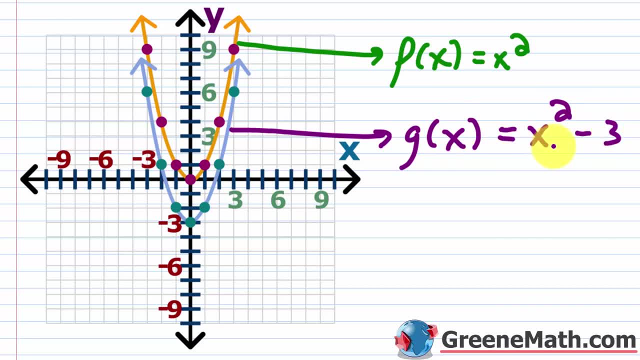 Okay. so if you wanted to graph g of x, if you got this on a test and they said: hey, graph x squared minus 3, you know that you just need to graph x squared and then just shift it down by 3 units. The easiest way to kind of do this is just to pick these points. 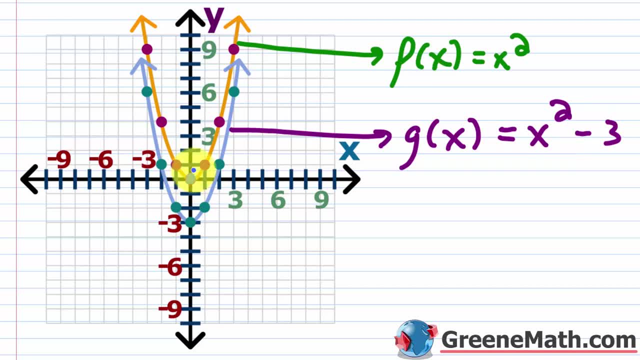 that you already know something like: let's say 0, 0, and say, okay, now it's going to be at 0, negative 3.. So that's my lowest point there, And then other points are just going. 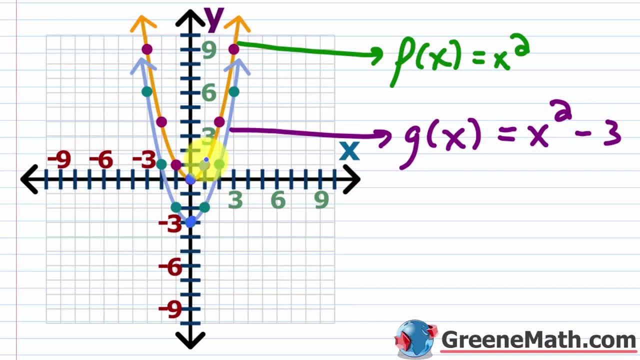 to be shifted down by 3 units. So something like 1, 1 is shifted down to 1, negative 3. Right, And so on and so forth, And that's how you would go about sketching your graph. But again, the reason this is happening is for a given x value. you now have a y value. 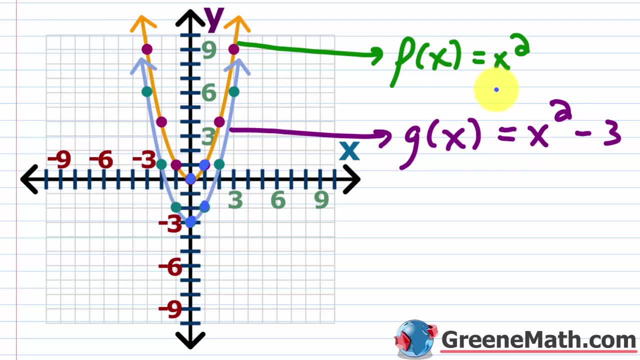 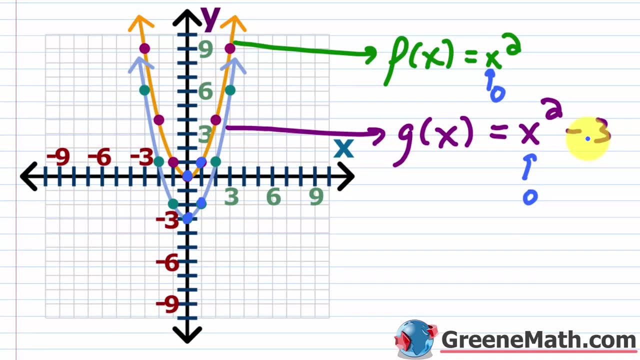 that's 3 units less. So again, for example, here, if I plug in a 0, I square it and I get 0.. Here, if I plug in a 0, I square it and I get 0.. But now I've got to subtract. 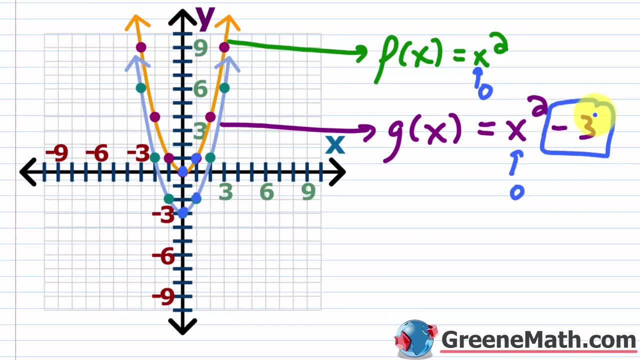 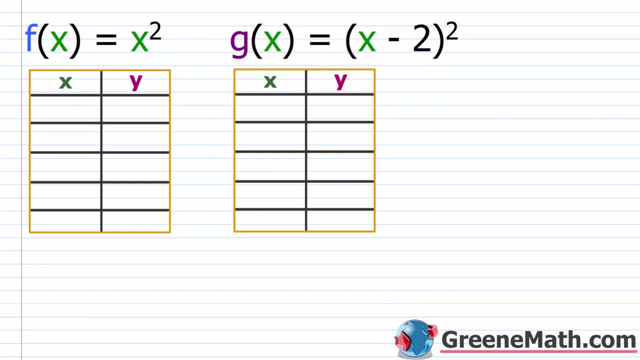 away 3.. I've got this extra step here, So I end up getting a y value of negative 3 or a y value that is 3 units. All right, Now let's consider something that is a little bit more challenging. What I just 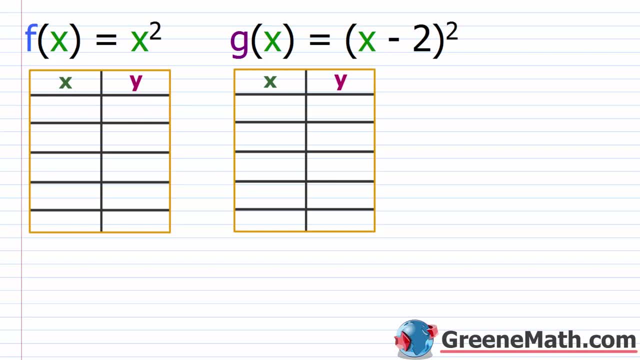 showed you was very straightforward What I'm going to show you here. I'm going to pretty much tell you that everyone that sees this for the first time does struggle with it, including myself. It's something that takes a lot of practice to kind of get used. 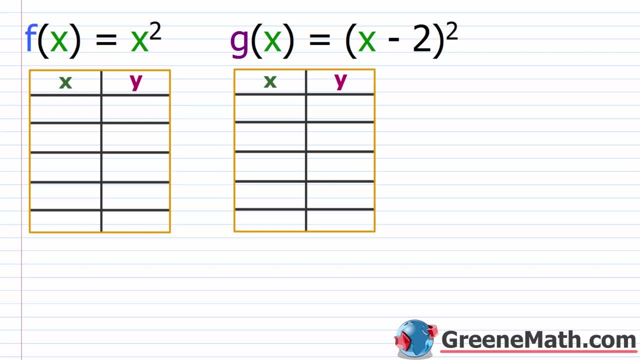 to Okay, And then the light bulb will go off for you, I promise, But when you first see it it is a bit confusing. Okay, So suppose we have f of x equals x squared and g of x is now equal to the quantity x. 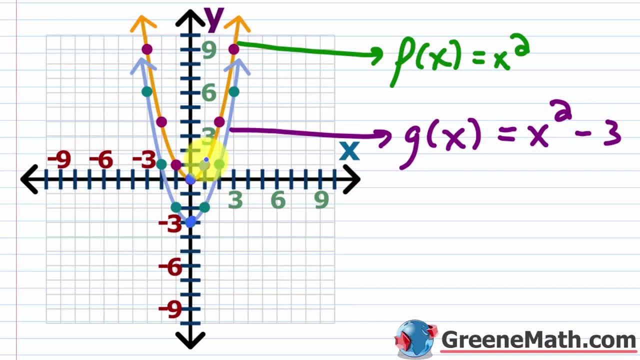 to be shifted down by 3 units. So something like 1, 1 is shifted down to 1, negative 3. Right, And so on and so forth, And that's how you would go about sketching your graph. But again, the reason this is happening is for a given x value. you now have a y value. 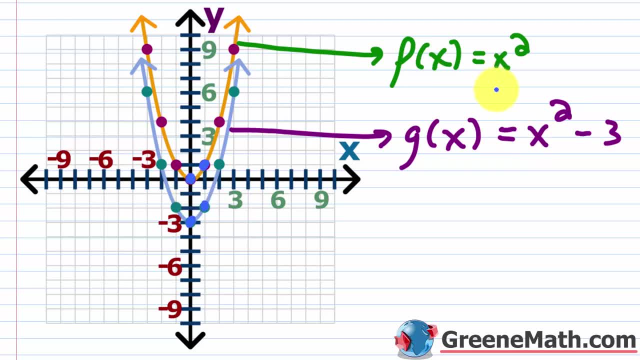 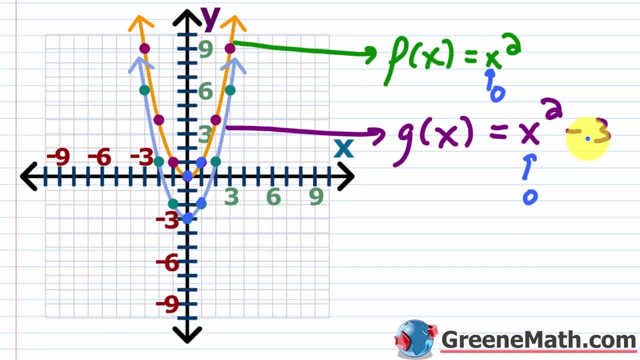 that's 3 units less. So again, for example: here, if I plug in a 0, I square it and I get 0.. Here, if I plug in a 0, I square it and I get 0, but now I've got a subtract away. 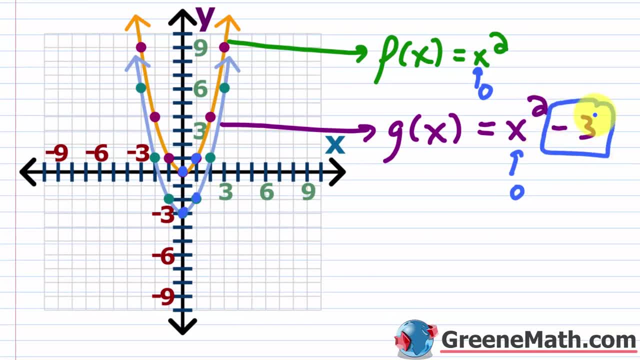 3.. I've got this extra step here, So I end up getting a y value of negative 3, or a y value that is 3 units less. So I'm actually going to get a y value of negative 3,, but I'm actually 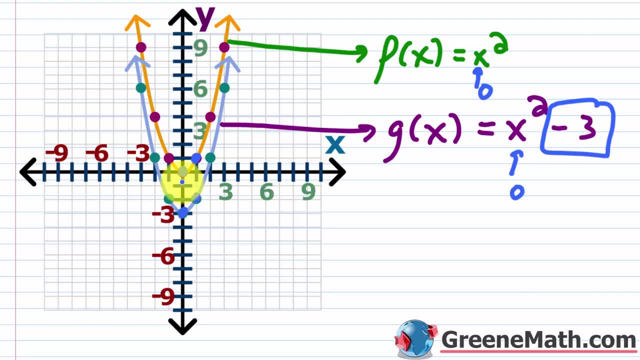 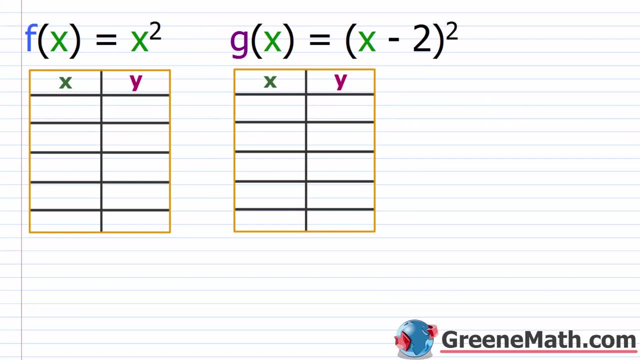 less for that, given x value. so that's why all these points are being shifted down by three units. all right, now let's consider something that is a little bit more challenging. what i just showed you was very straightforward. what i'm going to show you here, i'm going to pretty much tell you that. 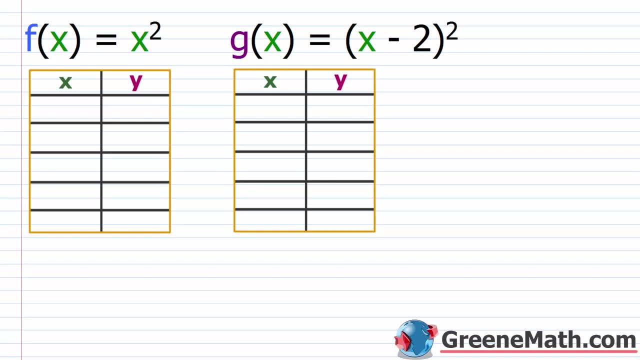 everyone that sees this for the first time does struggle with it, including myself. it's something that takes a lot of practice to kind of get used to. okay, and then the light bulb will go off for you, i promise, but when you first see it it is a bit confusing. so suppose we have f of x equals x. 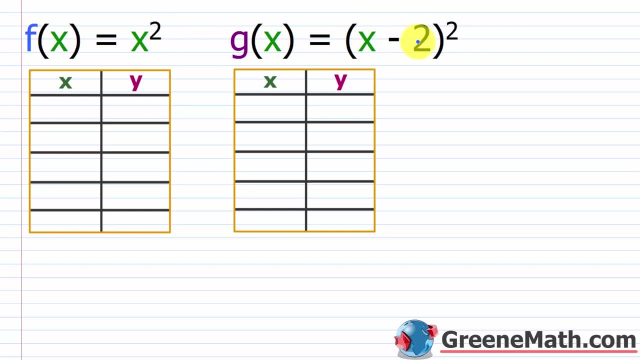 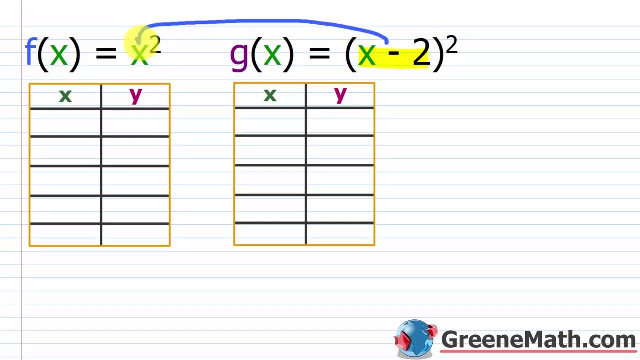 squared, and g of x is now equal to the quantity x minus two squared. so if we really think about it, this right here could be plugged in for x in f of x. okay, so i could really define g of x as being equal to f of x minus two, if i wanted to right, because if i plugged in an x minus two, 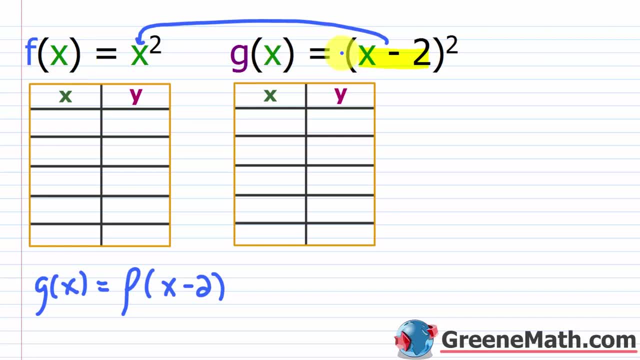 in for x and f of x, i would have this g of x, which is again the quantity x minus two squared. okay, so now that we know how to define that, let's think about what's going to happen. so let's start with these points. here we have kind of negative two four. we have negative one one. we have zero zero one one. 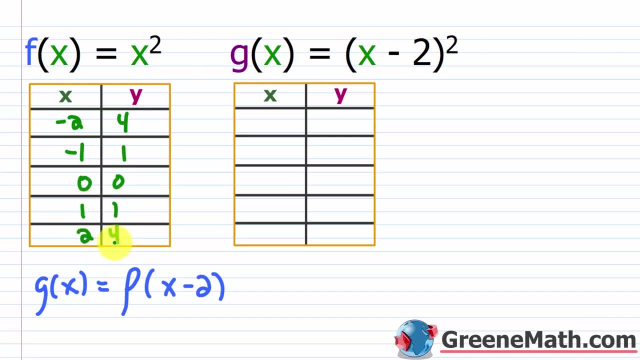 and we have two, four now. what do you think's going to happen? a lot of people think that this minus two here okay, this minus two here because it's associated with x. they think that everything's going to shift to the left by two units. right because the x values are occurring on. 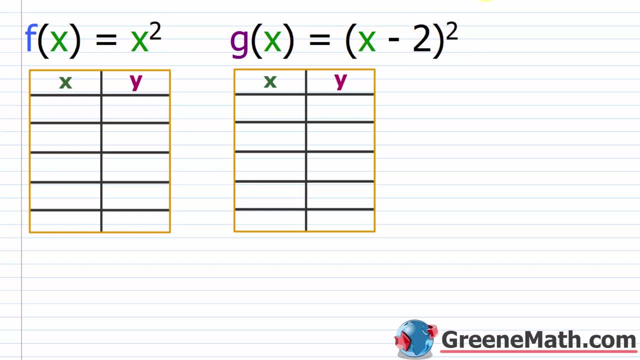 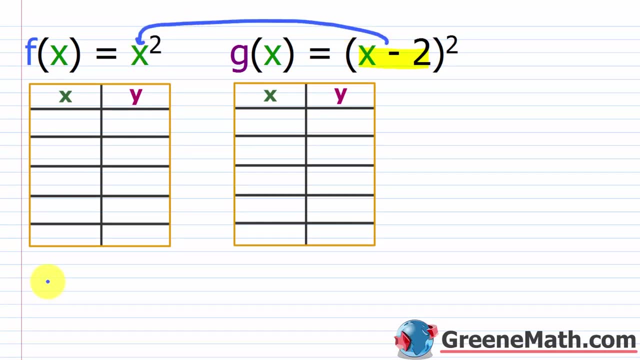 minus 2 squared. So if we really think about it, this right here could be plugged in for x in f of x. Okay, So I could really define g of x as being equal to f of x minus 2 if I wanted to Right, Because if I plugged in an x minus 2 in for x in f of x, I would have. 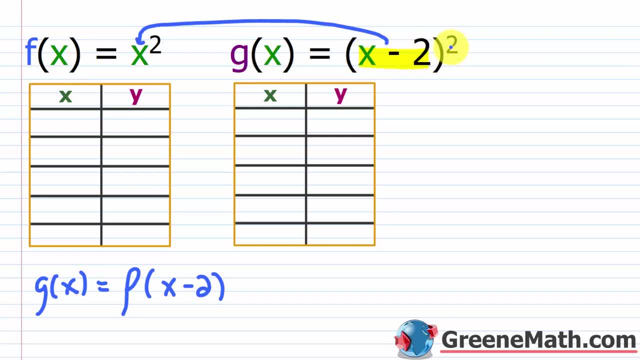 this g of x, which is again the quantity x minus 2 squared. Okay. so now that we know how to define that, let's think about what's going to happen. So let's start with these points here. We have kind of negative 2, 4.. We have negative 1, 1.. We have 0, 0, 1, 1, and we have 2, 4.. 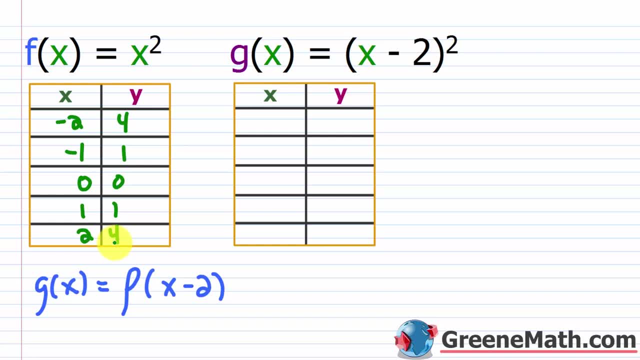 Now what do you think is going to happen? A lot of people think that this minus 2 here okay. this minus 2 here, because it's associated with x. they think that kind of everything's going to shift to the left by 2 units right, Because the x values are occurring on the 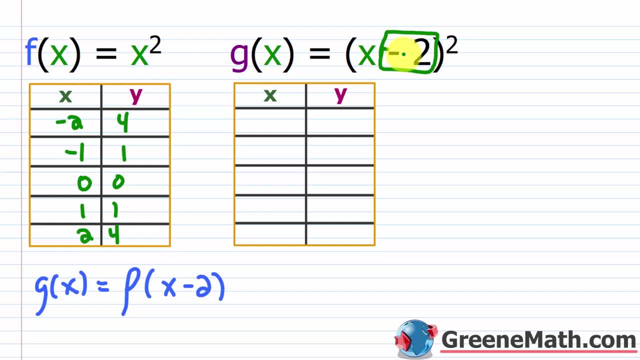 horizontal axis. So if we think about minus 2 horizontally, we intuitively feel like this should go to the left 2 units, But what's going to happen is it's actually going to go to the right by 2 units. okay, So let me fill in this table real quick and then I'll explain why. 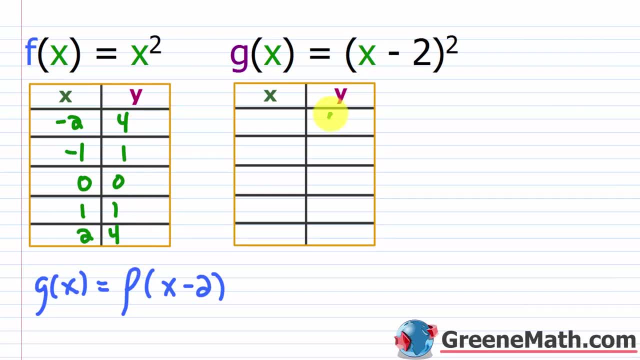 So for a given y value, okay, for a given y value. so 4, 1,, 0, 1, and 4, these x values are now going to be 2 units larger, okay? So instead of negative 2, it would be 0.. Instead of negative 1, it would be positive 1.. Instead of 0,, it would. 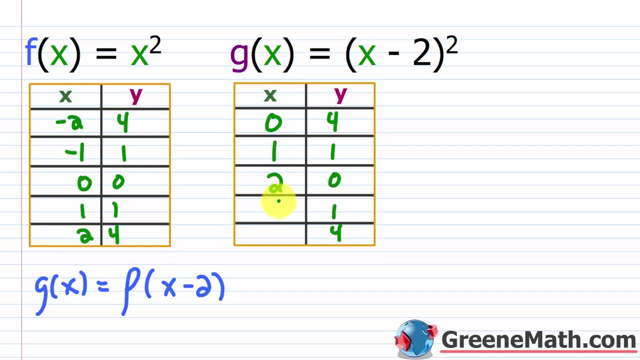 be 2.. Instead of positive 1, it would be 3., And then, instead of positive 2, it would be 4.. Now, if you want to check this, you can: 0 minus 2 is negative 2, negative 2 squared. 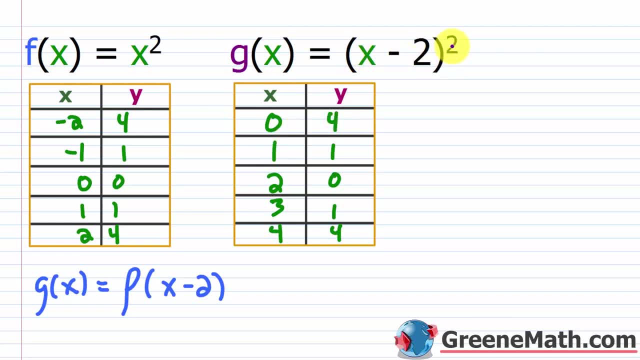 is 4.. So that one's good 1 minus 2 is negative 1, negative 1 squared is 1, that's good. 2 minus 2 is 0, 0 squared is 0, that's good. 3 minus 2 is 1, 1 squared is 1, that's good. And 4 minus 2 is. 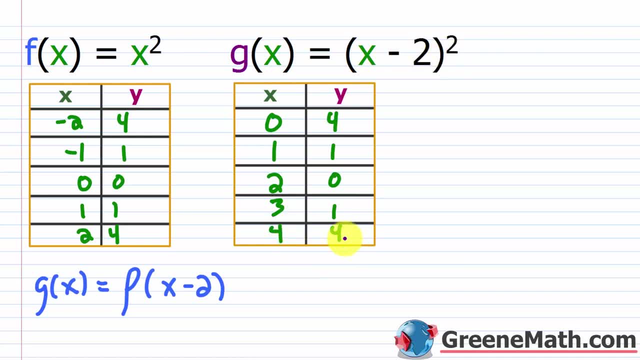 2, 2 squared is 4, that's good. So for a given y value, right? these y values are the same. the x values have been increased by 2 units. okay, So let's think about what's going on here. 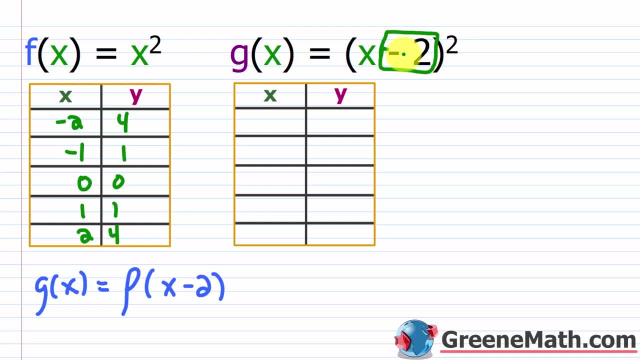 the horizontal axis. so if we think about minus two horizontally, we intuitively feel like this should go to the left two units, but what's going to happen is it's actually going to go to the right by two units. okay, so let me fill in this table real quick and then i'll explain why. so for a 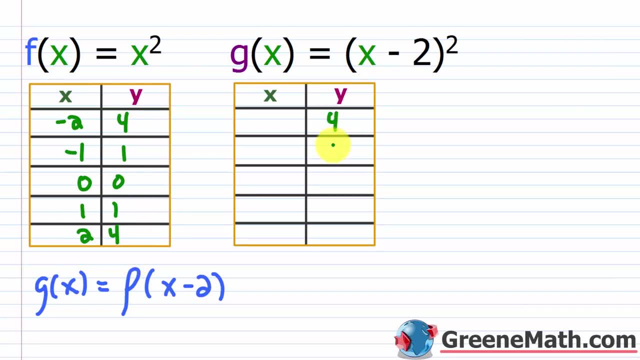 given y value. okay for a given y value. so four, one, zero one and four. these x values are going to be two units larger, okay, so instead of negative two, it would be zero. instead of negative one, it would be positive one. instead of zero, it would be two. instead of positive one, it would be three, and then. 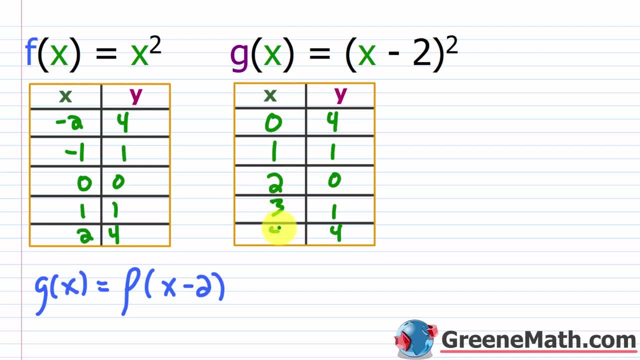 instead of positive two, it would be four. now, if you want to check this, you can. zero minus two is negative, two negative two squared is four, so that one's good, one minus two is negative, one negative. one squared is one. so we can't check this right now, so we're going to go ahead and let's see how we become. 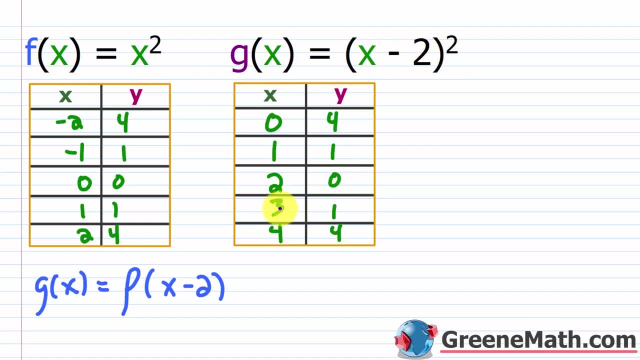 that's good. 2 minus 2 is 0, 0 squared is 0,. that's good. 3 minus 2 is 1, 1 squared is 1, that's good. And 4 minus 2 is 2, 2 squared is 4, that's good. So for a given y value, 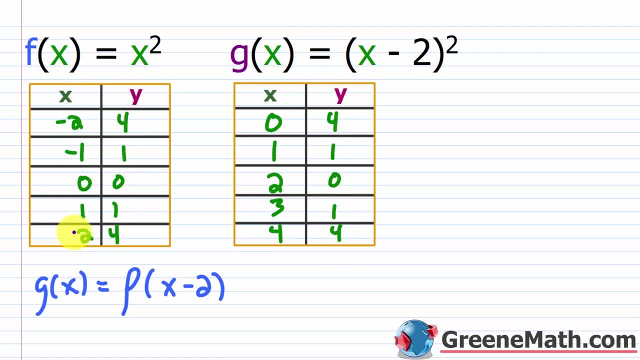 right, these y values are the same. the x values have been increased by 2 units. okay, So let's think about what's going on here. Well, what's happening is I'm plugging in something for x and then I'm subtracting away 2 before I square it. So what that means is that, in order. 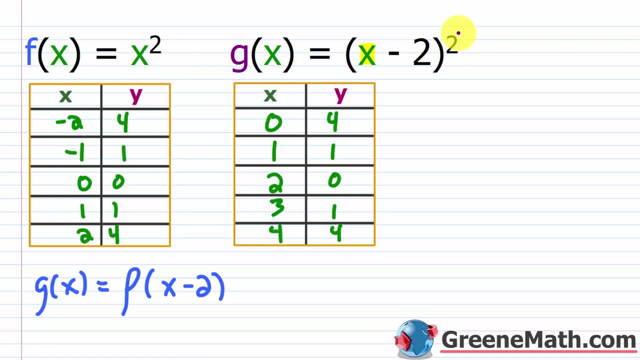 to obtain the same y value, my x value now needs to be 2 units larger, right, Because I have to undo what's being done to x, And that's going to be a key thing that comes up over and over in this lesson. So you want to remember that You need to think about what undoes what's being done. 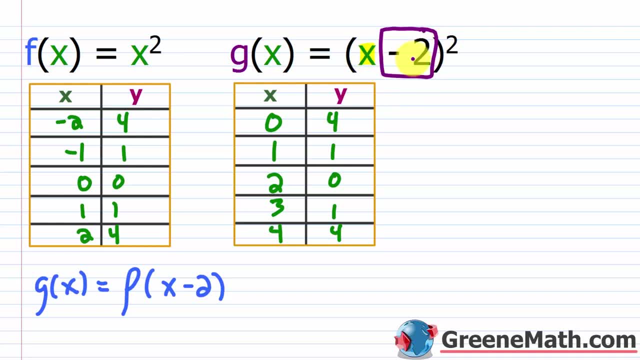 to x, Because I'm subtracting away 2 from x. for a given x value I subtract away two, So I'm really getting a y value that would have occurred with an x value kind of two units ago. if I'm thinking about in the f of x function, If I'm thinking about 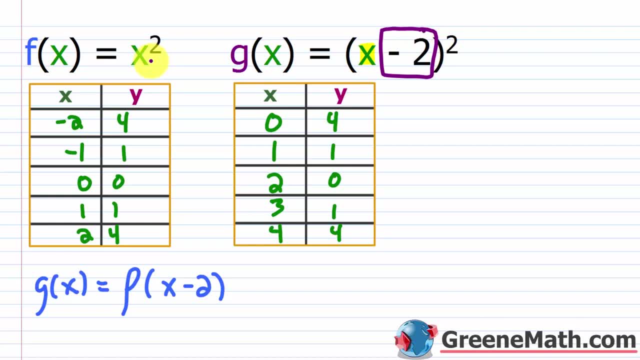 maintaining the same y value, then x now has to be two units larger to undo that minus two. And again, I know this is super confusing when you first hear it, But let's go ahead and look at the graph and see if it makes a little bit more sense. So I've graphed these already. kind of side. 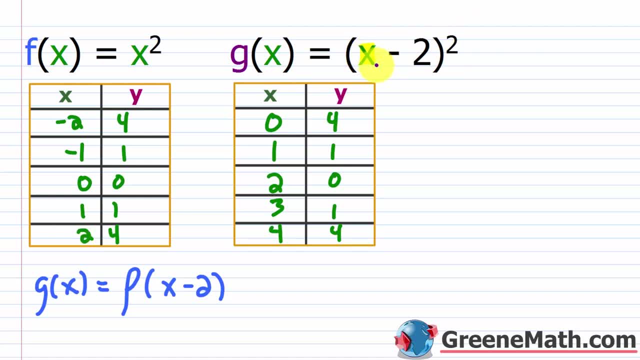 Well, what's happening is I'm plugging in something for x and then I'm subtracting away 2 before I square it. So what that means is that, in order to obtain the same y value, my x value now needs to be 2 units larger. right, Because I have to undo. 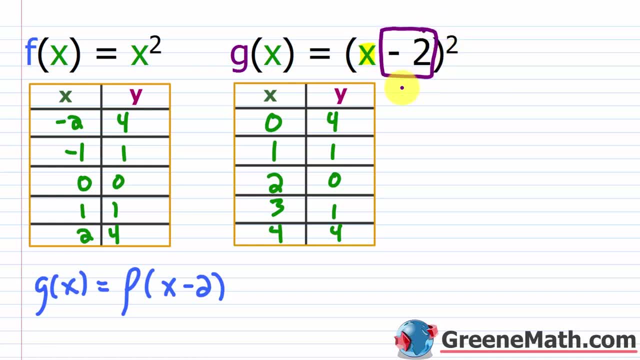 what's being done to x, And that's going to be a key thing that comes up over and over in this lesson. So you want to remember that. You need to think about what undoes what's being done to x, Because I'm subtracting away 2 from x for a given x value. 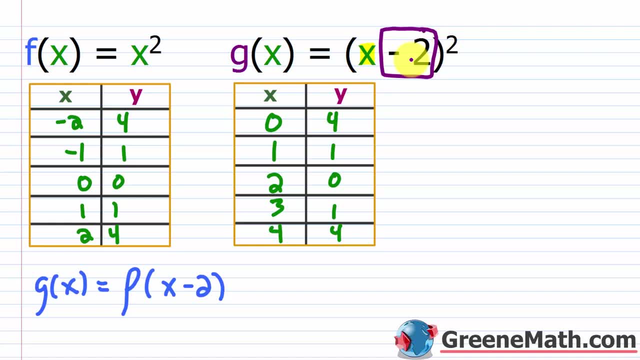 I subtract away 2, so I'm really getting a y value that would have occurred with an x value kind of 2 units ago. if I'm thinking about in the f of x function, If I'm thinking about maintaining the same y value, then x now has to be 2 units larger to undo that minus 2.. And again, 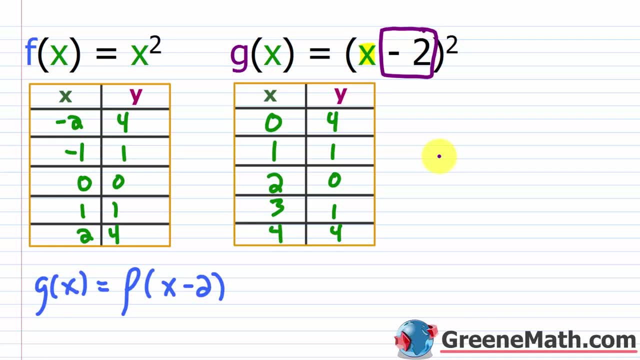 I know this is super confusing when you first hear it, but let's go ahead and look at the graph and see if it makes a little bit more sense. So I've graphed these already kind of side by side. So once again, the orange one. 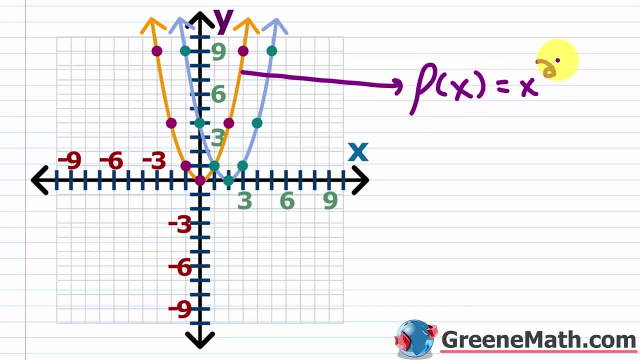 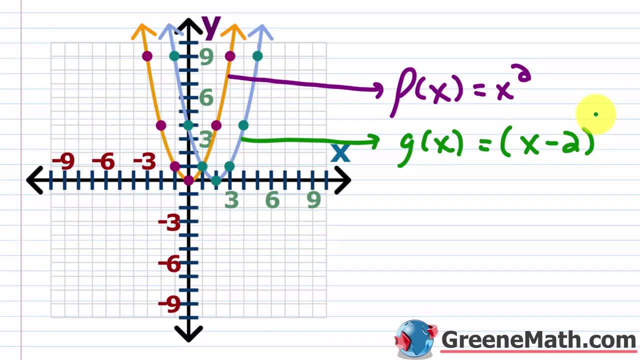 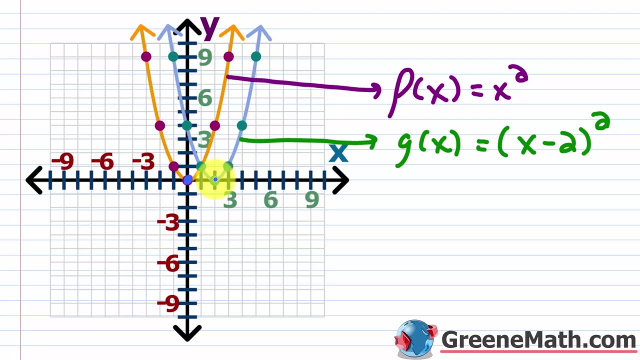 is my original f of x equals x squared, And my guy in light blue here is my g of x, which is the quantity x minus 2 squared. So again what you can see if I focus on this point: 0, 0,. it's been shifted 2 units to the right and now it's going to be at 2, 0.. Okay, let's think. 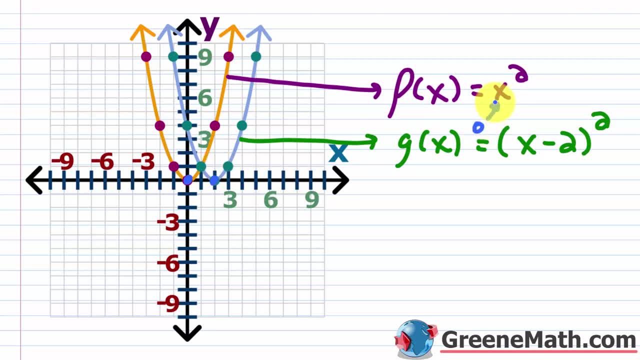 about y. Here I could plug in a 0 for x and I would get a 0 for y or f of x Here. if I plug in a 0 for x, what happens? Well, essentially I have negative 2, right, And then negative 2. squared is going to give me 4.. 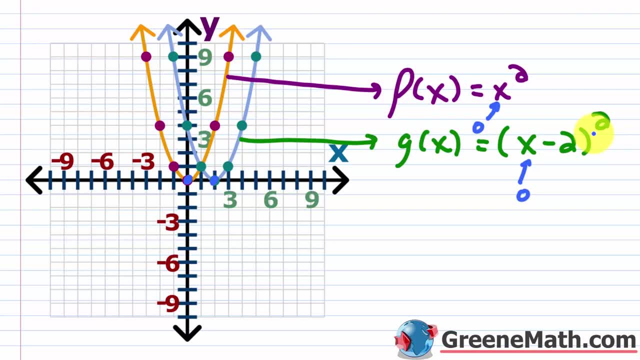 So that no longer works. That doesn't give me a y value of 0 anymore. In order to get a y value of 0, x now has to be 2 units larger than it was before to undo this. So now I need to plug in a. 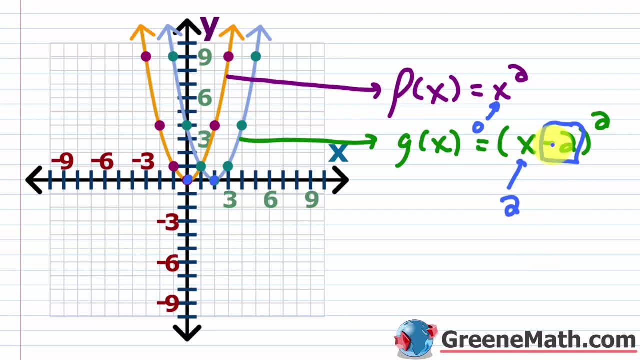 2 there. Okay, 2 minus 2 would give me 0.. 0 squared is 0.. So what happens is, for that same vertical value, that same value, I'm going to have to plug in a 2.. And I'm going to have to plug in a 2.. And 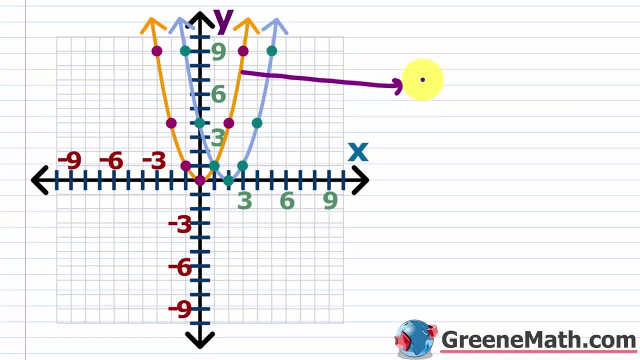 by side. So once again, the orange one. the orange one is my original f of x equals x squared, And my guy in light blue here is my g of x, which is the quantity x minus two squared. So again what you. 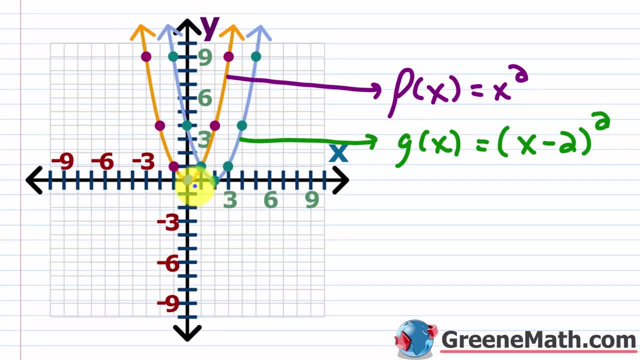 can see if I focus on this point: zero comma zero. it's been shifted two units to the right And now it's going to be at two comma zero. Okay, let's think about why. Here I could plug in a zero for. 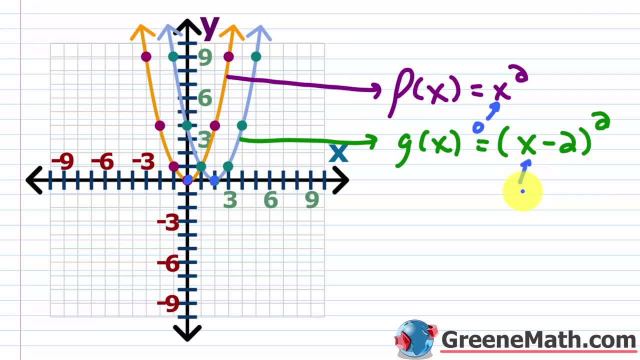 x and I would get a zero for y or f Here. if I plug in a zero for x, what happens? Well, essentially I have negative two right And then negative two squared is going to give me four, So that no longer works. That doesn't give. 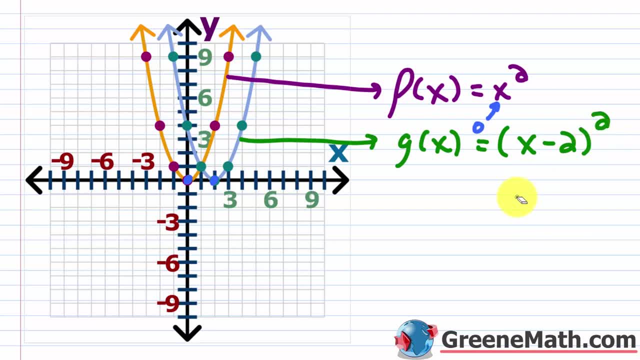 me a y value of zero anymore. In order to get a y value of zero, x now has to be two units larger than it was before to undo this. So now I need to plug in a two there. Okay, two minus two would. 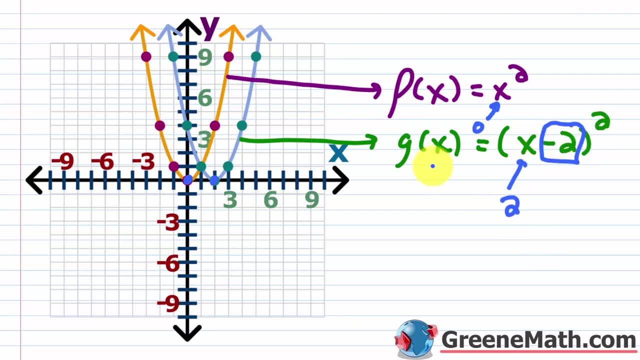 give me zero. zero squared is zero. So what happens is, for that same vertical value, that same y value of zero, x now had to be moved two units to the right. So what happens is everywhere on that graph is going to be shifted. 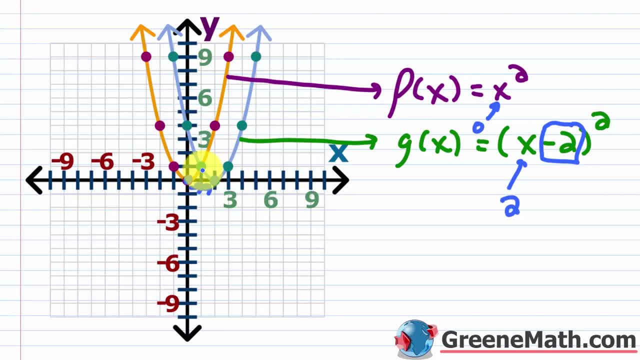 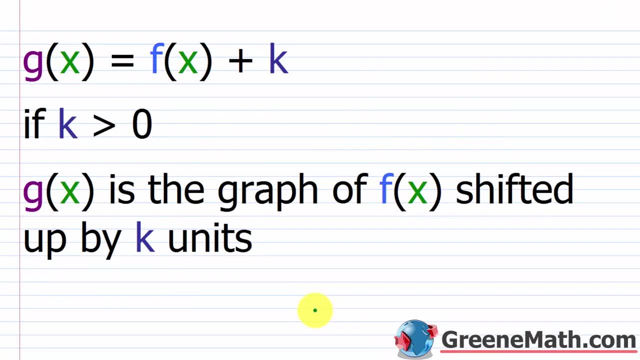 two units to the right Because again for that same y value, x now has to be two units larger again to undo this minus two right here. All right, let's go through kind of the textbook definition of this. This is something you're going to get in your course And it's confusing a lot of. 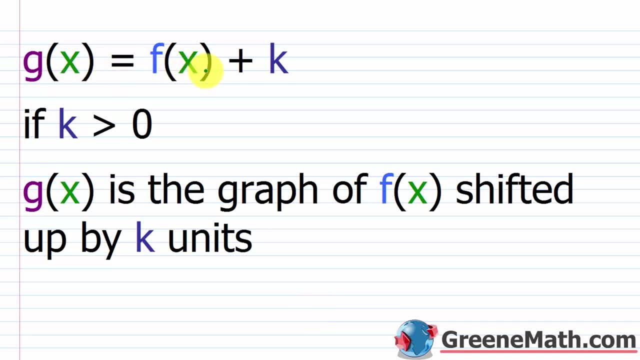 time. So I want to plug in a two here, And then negative two squared is going to give me four. So break this down. So we have g of x equals f of x plus k, And the first situation is we say: if k is, 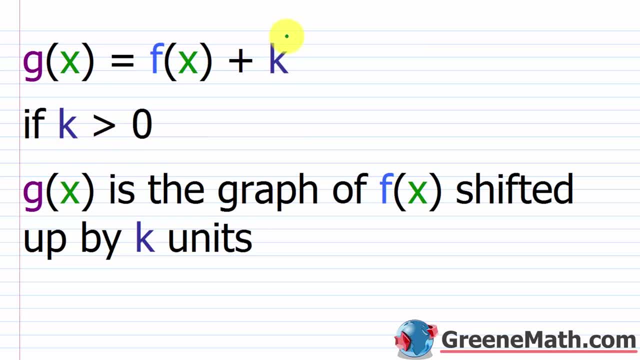 greater than zero. So if k is some positive real number, that's all we're saying. So if this guy is a positive real number, then g of x is just the graph of f of x shifted up by k units. This is completely logical. it should make sense for you. For an example, let's just say f of x is again x. 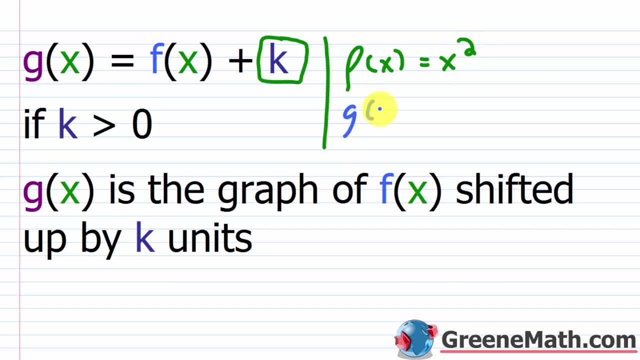 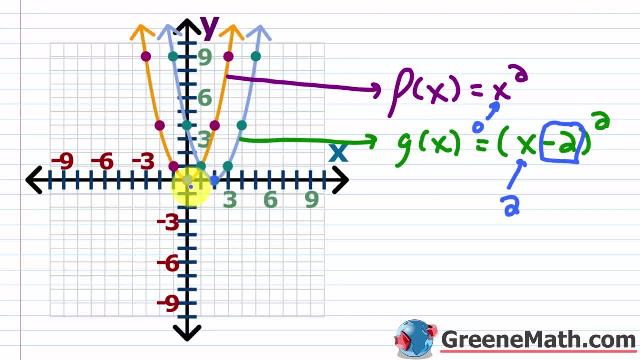 plug in a 2.. And I'm going to have to plug in a 2. And I'm going to have to plug in a 2. And I'm going. y value of 0, x now had to be moved 2 units to the right. So what happens is everywhere on that. 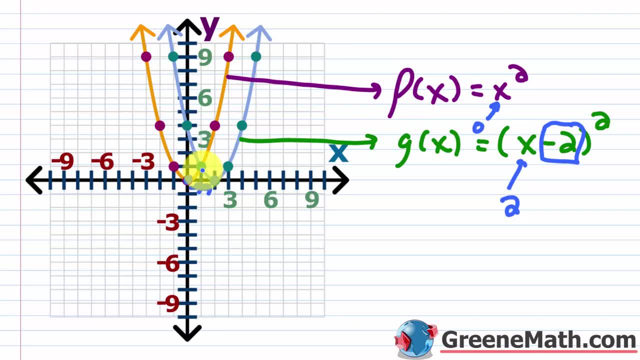 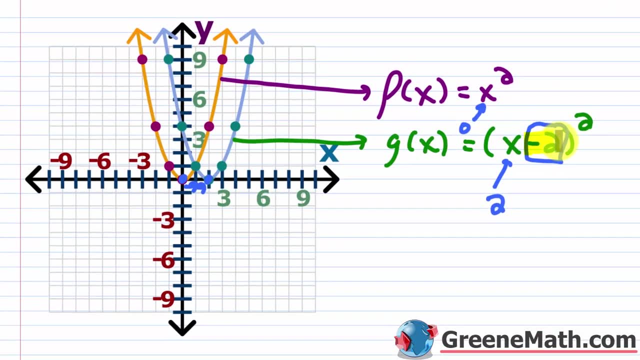 graph is going to be shifted 2 units to the right Because, again for that same y value, x now has to be 2 units larger again to undo this minus 2 right here. Alright, let's go through kind of. 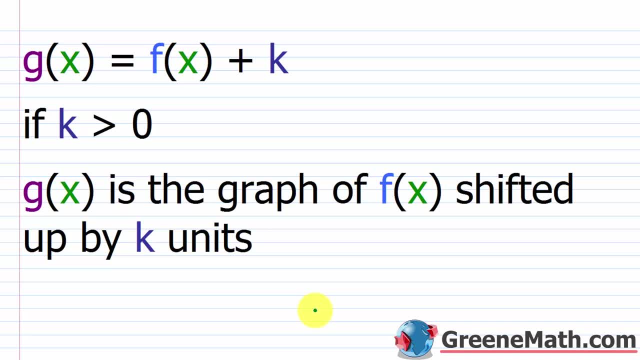 the textbook definition of this. This is something you're going to get in your course And it's confusing a lot of times, So I want to break this down. So we have g of x equals f of x plus plus k, and the first situation is we say: if k is greater than zero, so if k is some positive real. 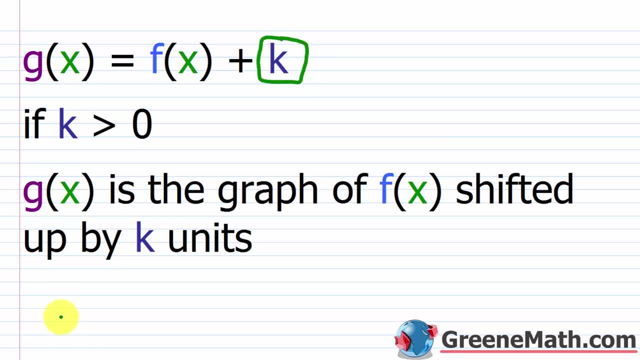 number. that's all we're saying. so if this guy is a positive real number, then g of x is just the graph of f of x shifted up by k units. this is completely logical. it should make sense for you. for an example, let's just say: f of x is again x squared. okay, something really easy. well, let's say: 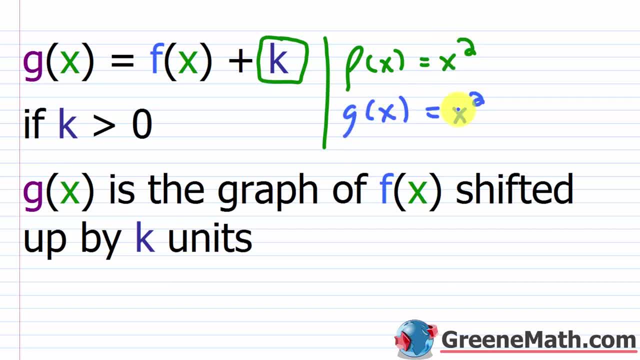 we had g of x and this is x squared, so this part's the same, and then plus some positive number, let's just call it 13, okay. so we should know by looking at that instantly that g of x is essentially just the graph of f of x. it's x squared, just shifted up by 13 units. right, because for any given x value, 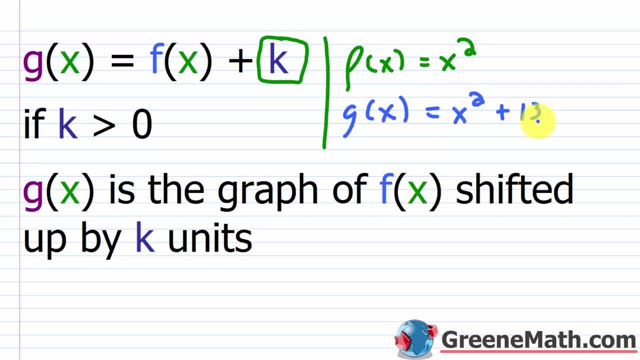 you're going to plug it in, you're going to square it and then you're going to add 13 to the result. so the y value is going to increase by 13. so every point in that graph of f, of x, moves up 13 units if 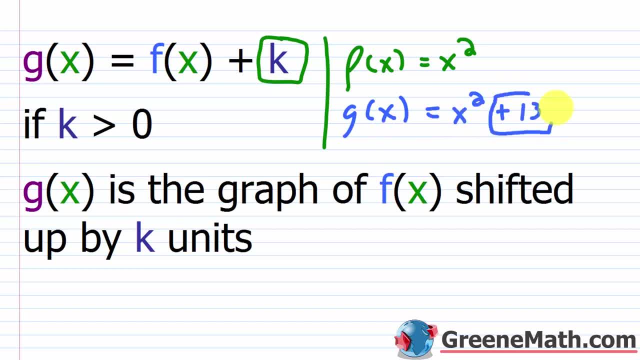 you're going to graph g of x. okay, that's all this plus 13 is doing. so later on we're going to hear this inside the function, outside the function. this is happening outside the function. okay, you have your f of x. nothing's being done to that, it's outside. so you have the plus k happening on the. 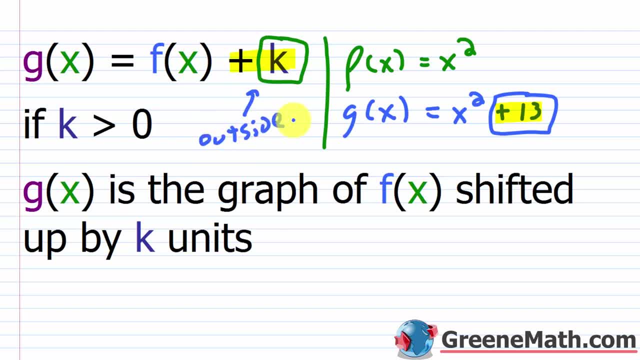 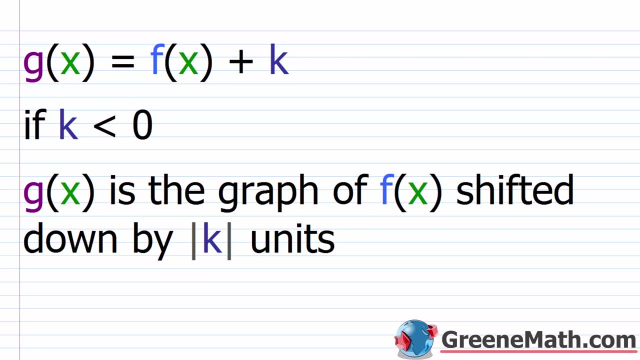 outside. let me write that. so this is the outside of the function. if something happens to the outside of the function, it's a vertical shift, okay. what happens inside? it's a horizontal shift. now you also have the case where you're shifting down- okay, and we also saw an example of this earlier. 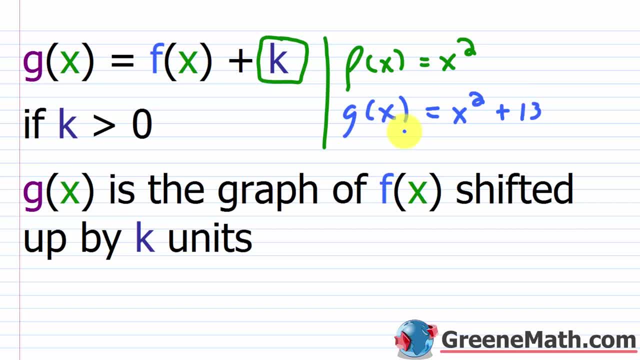 looking at that instantly, that g of x is essentially just the graph of f of x. it's x squared, just shifted up by 13 units. right? Because for any given x value, you're going to plug it in, you're going to square it and then you're going to add 13 to the result. So the y 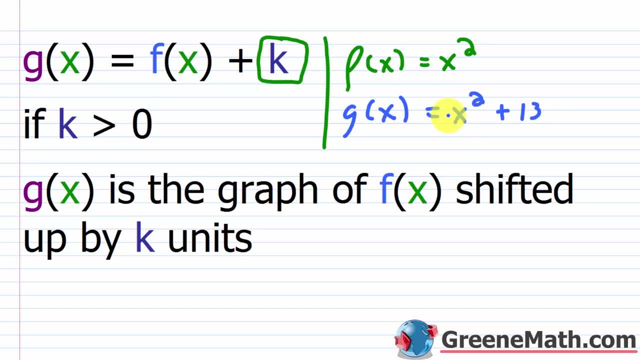 value is going to increase by 13.. So every point in that graph of f of x moves up 13 units. if you're going to graph g of x, okay, that's all you're going to do. So you're going to add 13 to. 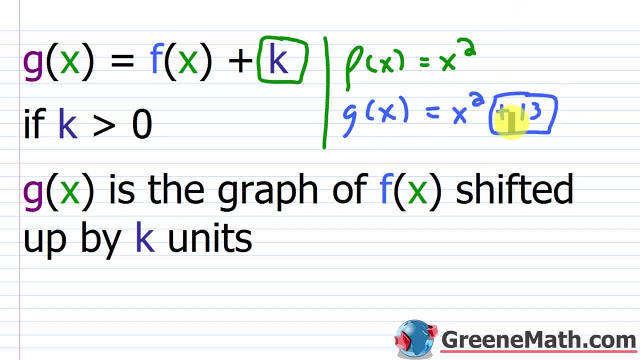 all this plus 13 is doing. So later on you're going to hear this inside the function, outside the function. this is happening outside the function. okay, you have your f of x. nothing's being done to that, it's outside. So you have the plus k happening on the outside. let me write that. 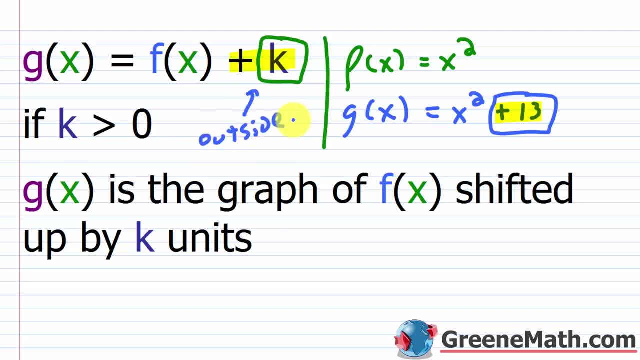 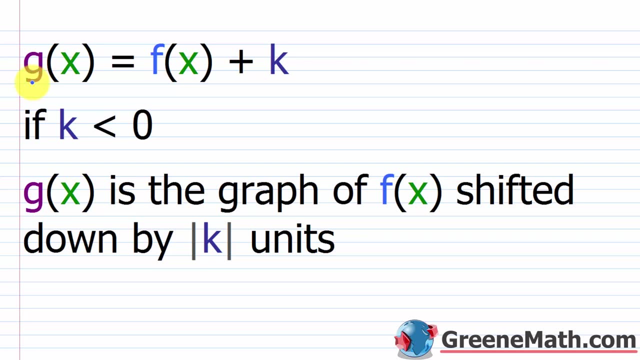 so this is the outside of the function. If something happens to the outside of the function, it's a vertical shift. okay, what happens inside, it's a horizontal shift. Now you also have the negative function. So if I have a value of x and I'm going to say let's look at the value of x, 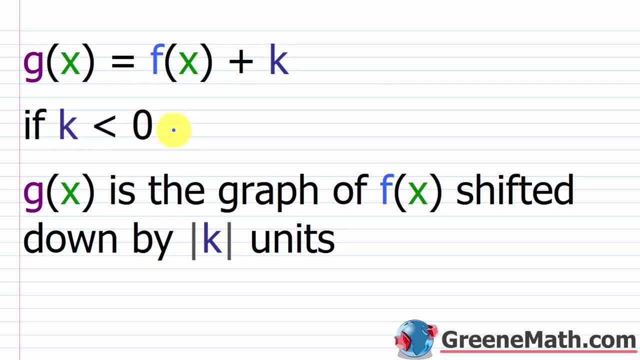 I'm going to say that we're going to have a negative function. So I'm going to say that we're going to have a negative function. So let's say that we're going to have a negative function. Now, the way this is written is a bit confusing, So let me explain that in a minute. For now, let's just 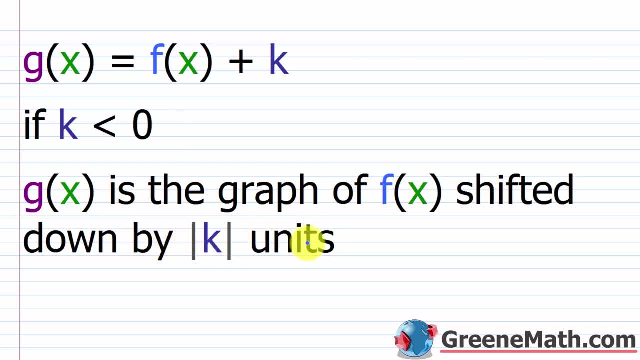 say that g of x is the graph of f of x shifted down by the absolute value of k units. So they just want to give you something. that's a generic rule. they don't cover kind of every scenario. Generally we don't write stuff as plus negative, we just write minus a number, okay. So for example, 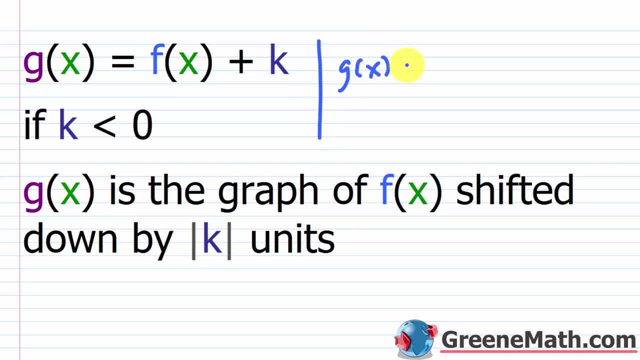 So, for example, earlier I gave you g of x was equal to x squared minus three. okay, So following this rule, I don't have plus some number, I have minus some number. So I would have to transform it and say this is plus a negative three, okay. 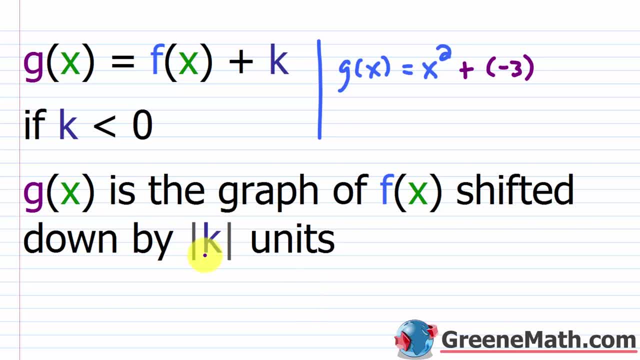 So we would say that the graph is shifted down: the absolute value of k in this case the absolute value of negative three. so it's shifted down by three units, But that's a bit of an overkill. What I would just say is: 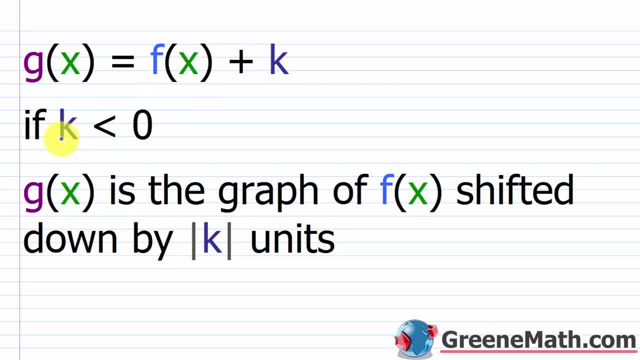 so we're going to say that g of x is equal to f of x plus k. now we're going to say that k is less than zero, so k is some negative number. now the way this is written is a bit confusing, so let me explain that in a minute. for now, let's just say that g of x is the graph of f of x shifted down. 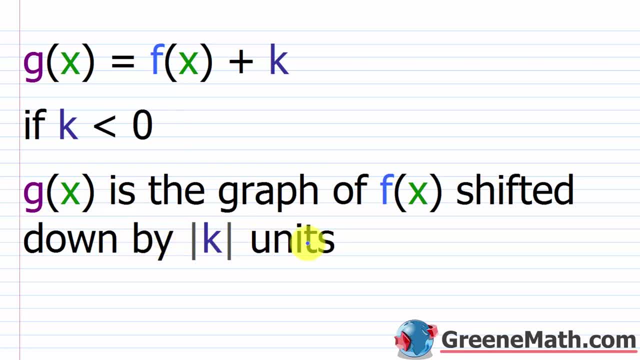 by the absolute value of k units. so they just want to give you something that's a generic rule. they don't cover kind of every scenario. generally we don't write stuff as plus negative, we just write minus a number, okay. so for example earlier i gave you g of x is equal to f of x plus k. so 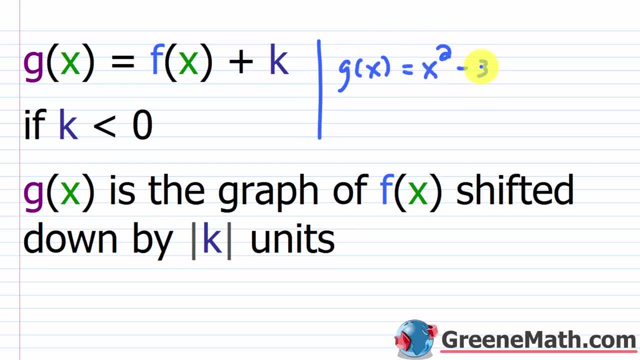 g of x was equal to x squared minus three. okay, so, following this rule, i don't have plus some number, i have minus some number. so i would have to transform it and say this is plus a negative three. okay, so we would say that the graph is shifted down: the absolute value of k, in this case the 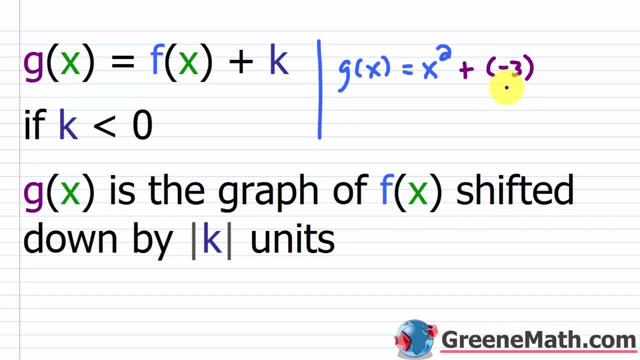 absolute value of negative three. so it's shifted down by three units, but that's a bit of an overkill. what i would just say is: if you're subtracting something away, so if you're subtracting away a positive number, so minus three here and you're subtracting something away- a positive number. 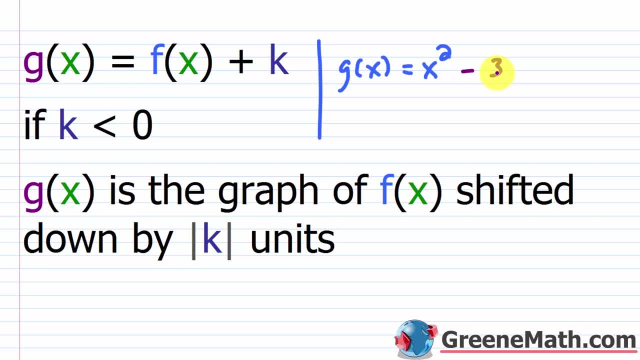 you should be able to look at that and say: well, i know that could be written as plus negative three. so i know i'm going to shift down by three units. so if it's minus a positive, then you're shifting down by this number of units. so if it was, let's say, h of x is equal to x squared minus 21. i know. 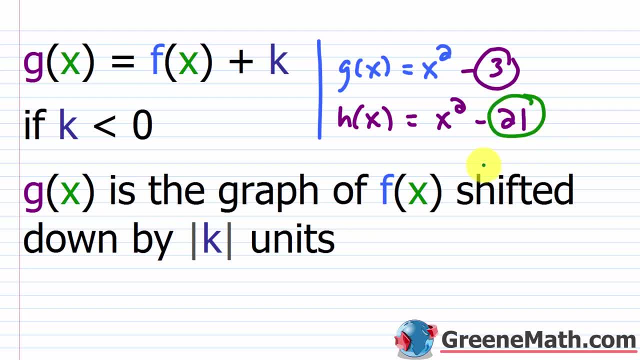 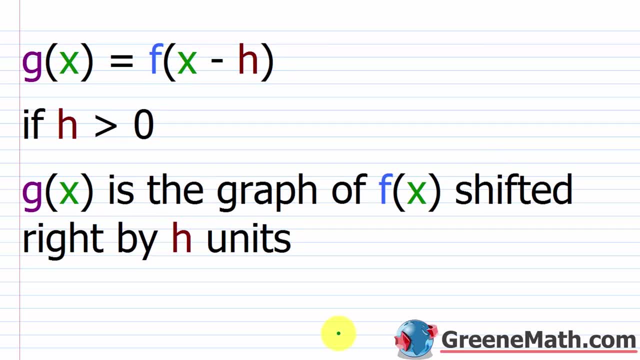 that again, i'm just going to shift down by this number of units. okay, that's all. it is all right. let's talk about the more difficult, the more challenging scenario, the one that everyone seems to you know not understand at first- again, including myself. the first time i saw this i was really confused. so let's say, g of x equals f of x. 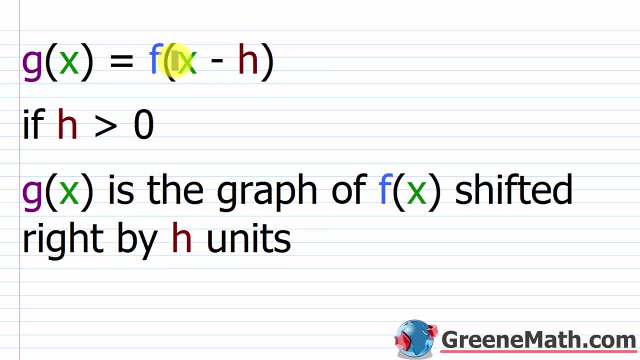 minus h. so now what's happening is our action is inside the function. i'm plugging something in for x, okay, so i'm plugging in the quantity x minus h in for x and f of x to get my g of x, okay, so if it's going on the inside, let me write that down. you got to be thinking horizontal shift, okay. 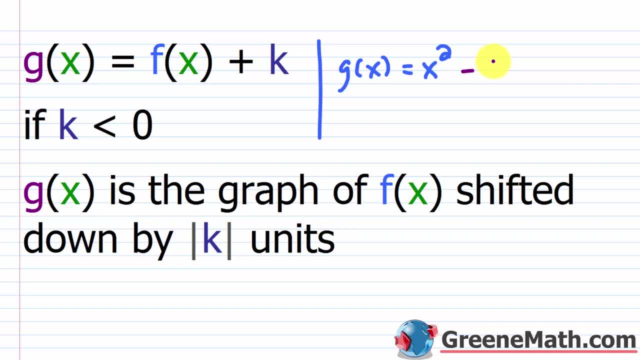 if you're subtracting something away. so if you're subtracting away a positive number, so minus three. here you should be able to look at that and say, well, I know that could be written as plus negative three. so I know I'm gonna shift down by three units. 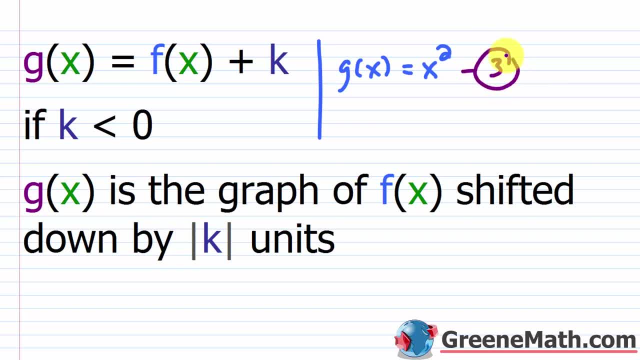 So if it's minus a positive, then you're shifting down by this number of units. So if it was, let's say, h of x is equal to x squared minus 21,. I know that again, I'm just gonna shift down by this number of units, okay. 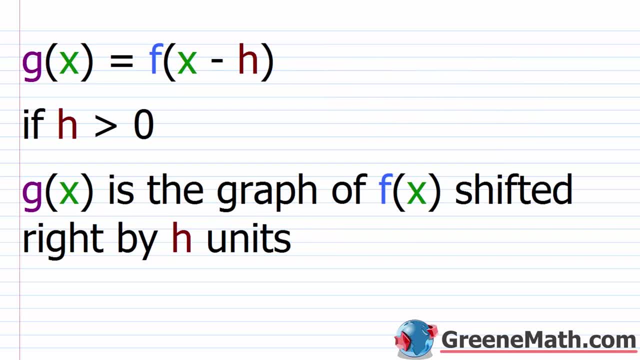 That's all. it is All right. let's talk about the more difficult, the more challenging scenario, the one that everyone seems to you know, not understand at first, again, including myself. The first time I saw this, I was really confused. 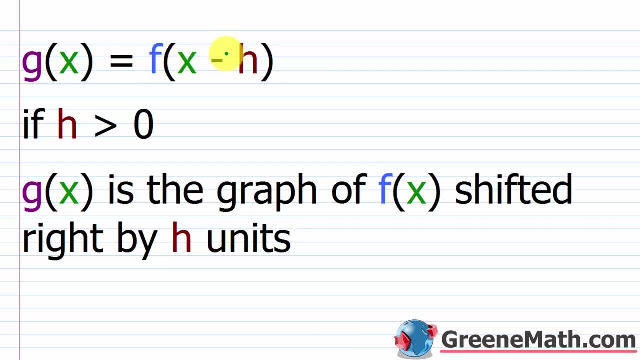 So let's say g of x equals f of x minus h. So now what's happening is our action is inside the function. I'm plugging something in for x, okay. So I'm plugging in the quantity x minus h in for x, in f of x, to get my g of x, okay. 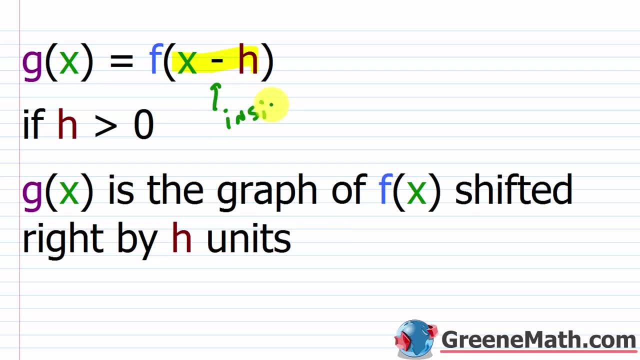 So if it's going on the inside, let me write that down. You've gotta be thinking horizontal shift, okay? So now if h is greater than zero, again this is the confusing part. g of x is the graph of f of x shifted right. 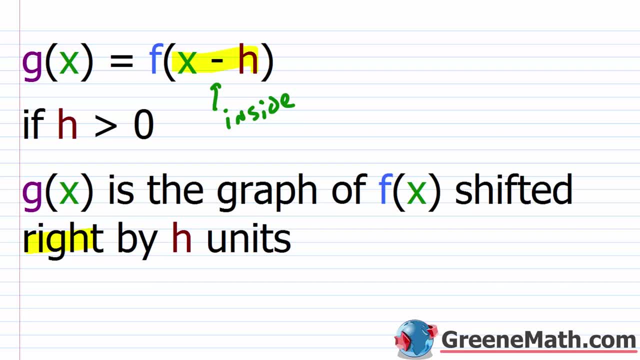 shifted right by h units. okay, So let's say that we had g of x was equal to the quantity, let's say x minus seven, and this is squared Again, a lot of people look at that and they say, okay, well, if my f of x is x squared. 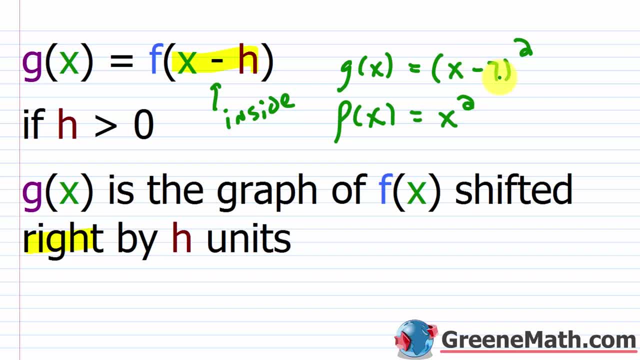 will my g of x. they'll say: okay, it's x minus seven, so I'm shifting to the left seven units. But that's wrong. okay, You've gotta shift to the right by seven units. And the reason for that? once again. 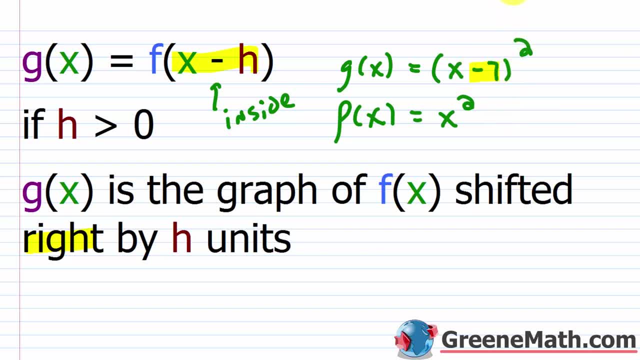 I've gotta always think about what's gonna undo, what's being done to x. That's really how you get your shift. You can use this rule if you want and you can say: okay, well, I know, in this case h is going to be seven, right? 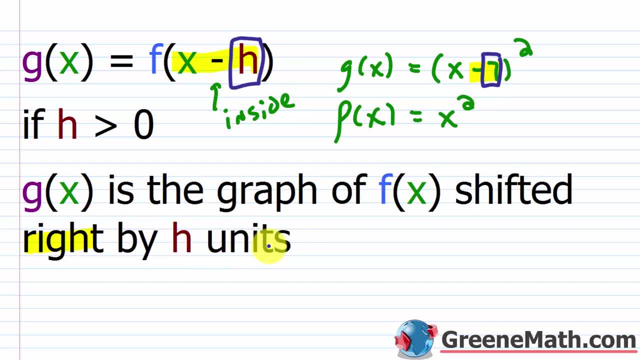 If you wanna match that up perfectly. And my rule said: hey, it shifts to the right by h units, so it shifts into the right seven units. You can get it that way. But the easiest way to think about it is just to say what undoes what's being done to x. 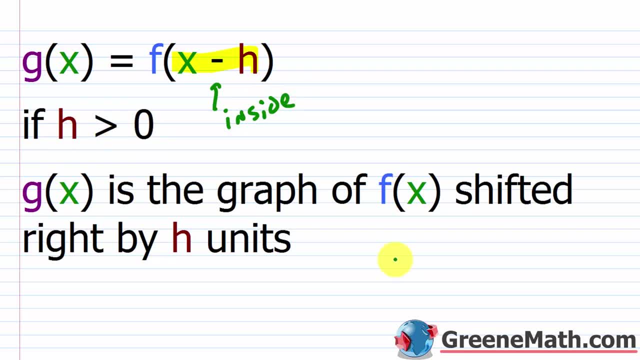 now if h is greater than zero. again, this is the confusing part. g of x is the graph of f of x shifted right, shifted right by h units. okay, so let's say that we had g of x was equal to the quantity. let's say x minus seven and this is squared. again, a lot of people look at that and 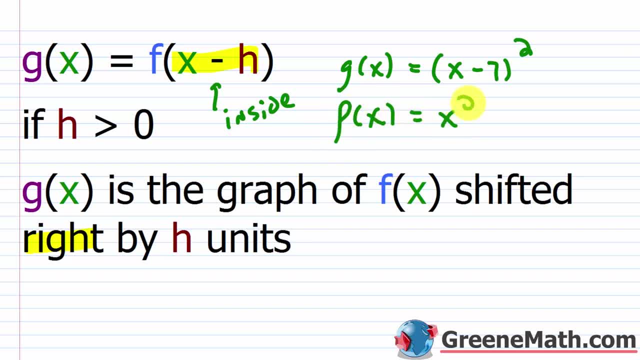 they say: okay, well, if my f of x is x squared, well, my g of x? they'll say: okay, it's x minus seven. so that's wrong. okay, you've got to shift to the right by seven units. and the reason for that? once again, i've got to always think about what's going to undo, what's being done to x. that's really. 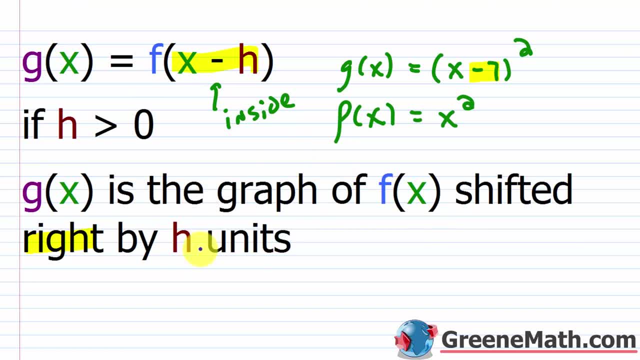 how you get your shift. you can use this rule if you want. you can say: okay, well, i know, in this case h is going to be seven, right, if you want to match that up perfectly? and my rule said: hey, it shifts to the right by h units, so it shifts into the right seven units. you can get it that way, but 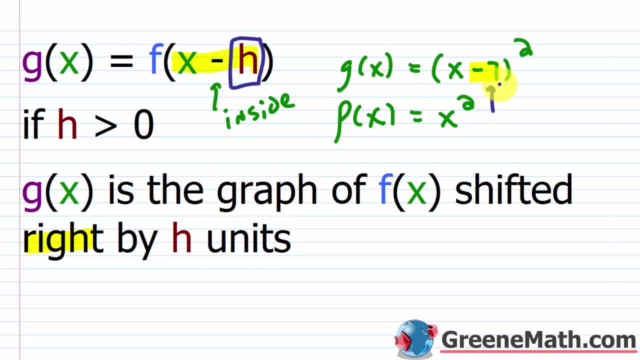 the easiest way to think about this is just to say what undoes what's being done to x and that's x. since what's being done to x is i'm subtracting away seven. to undo it i've got to add seven. so that tells me if i'm adding seven. on the horizontal axis, i'm moving to the right by seven units. 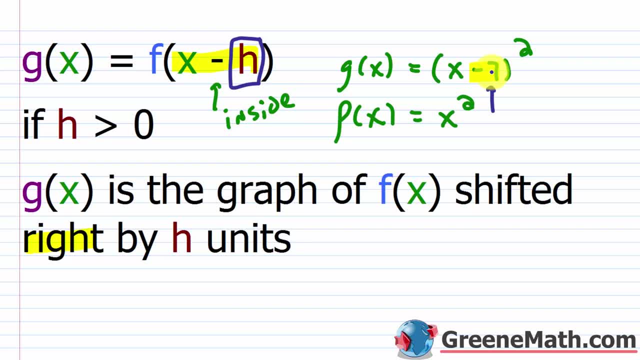 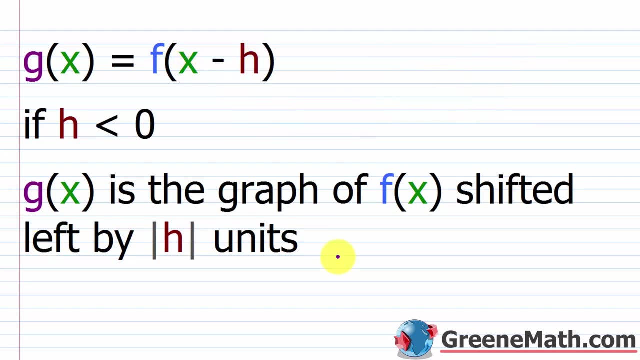 because to get the same y value, okay, now x has to be seven units larger, okay. so to maintain that vertical position, i've got to move seven units to the right on the x axis because i've got to undo that minus seven. okay, that's what's going on all right. now let's look at the more. 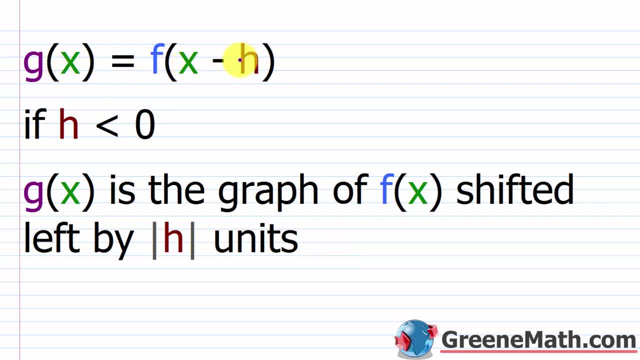 confusing rule. so we have: g of x equals f of the quantity x minus h. again, notice how we are plugging in for x and f of x. so this is on the inside. again, this is on the inside. and now we say: if h is less than zero, well, what's going to happen is g of x, is the graph of f of x shifted left? 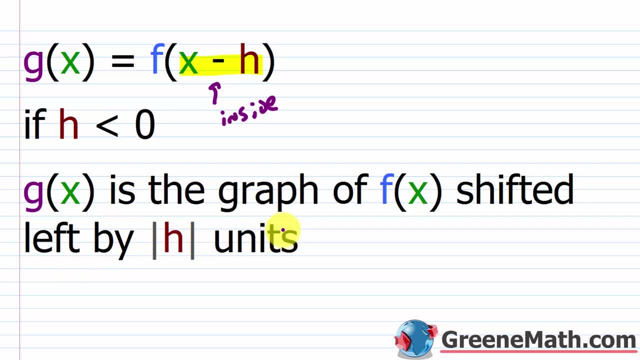 by the absolute value of h units. now this can be quite confusing, so let's break this down. so suppose we had g of x and it was equal to the quantity, let's say, x plus seven squared. well, we know at this point that minus a negative is. 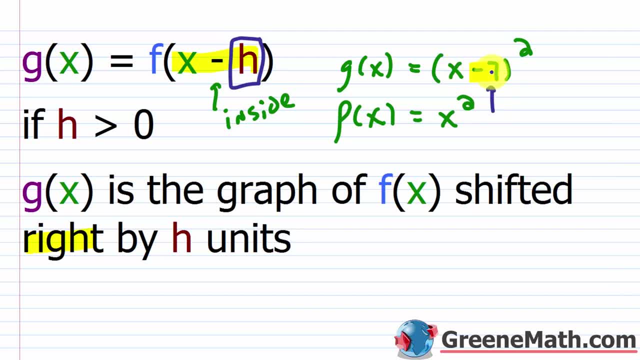 Since what's being done to x is I'm subtracting away seven. to undo it I've gotta add seven. So that tells me if I'm adding seven on the horizontal axis, I'm moving to the right by seven units, Because to get the same y value- okay. 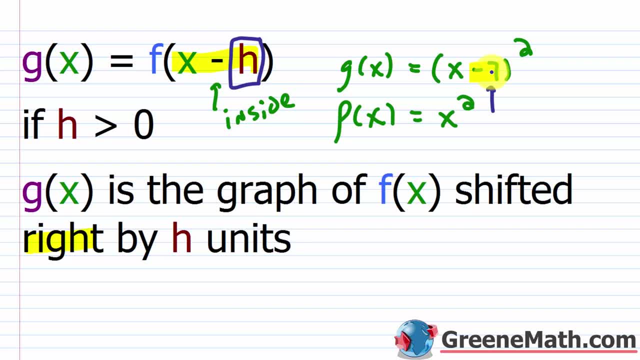 now x has to be seven units larger, okay. So to maintain that vertical position, I've gotta move seven units to the right on the x-axis because I've gotta undo that minus seven. okay, That's what's going on. 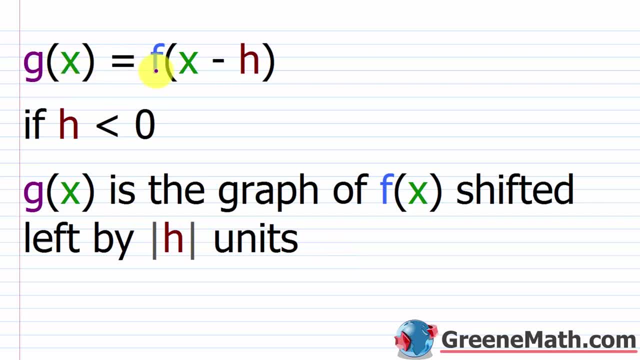 All right, now let's look at the more confusing rule. So we have: g of x equals f of the quantity x minus h. Again, notice how we are plugging in for x in f of x. So this is on the inside again. 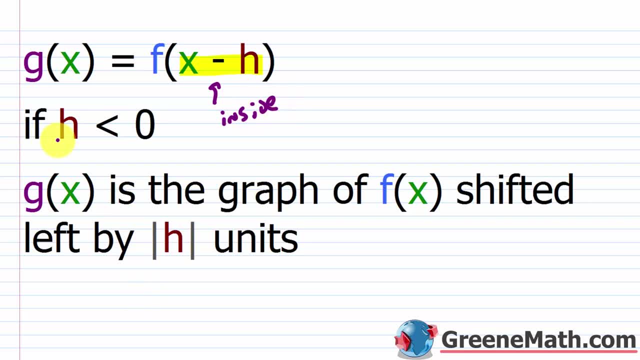 This is on the inside. And now we say: if h is less than zero, well, what's gonna happen is g of x is the graph of f of x shifted left by the absolute value of h units. Now this can be quite confusing. 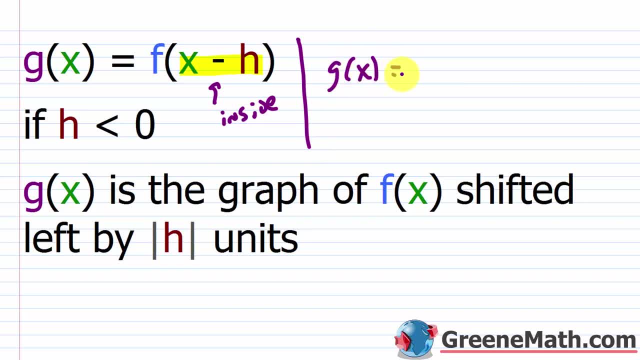 Let's take a look at this step. So suppose we had g of x and it was equal to the quantity, let's say x plus seven squared. Well, we know at this point that minus a negative is plus a positive, So you gotta be thinking this way. 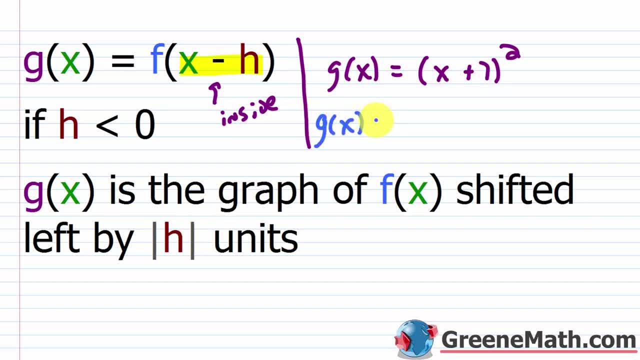 that to write it like this and follow this rule, I would say: g of x is equal to the quantity x minus a negative seven and that amount squared. So, following this, let me just kind of erase this real quick. Following this, I've got my minus and I've got my minus. 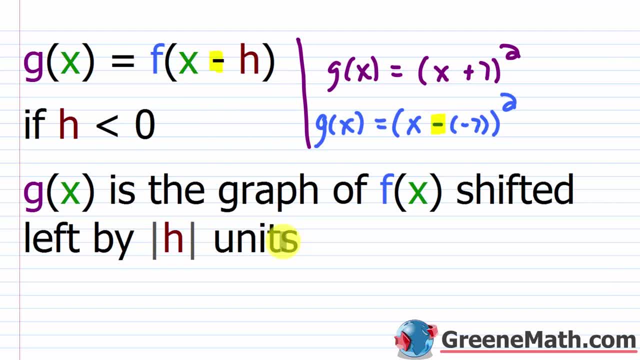 So I've written it perfectly in line with the formula they've given me. So I know that h now is going to be negative seven. Okay, h is negative seven. So just following the rule g of x, is the graph of f of x shifted left. 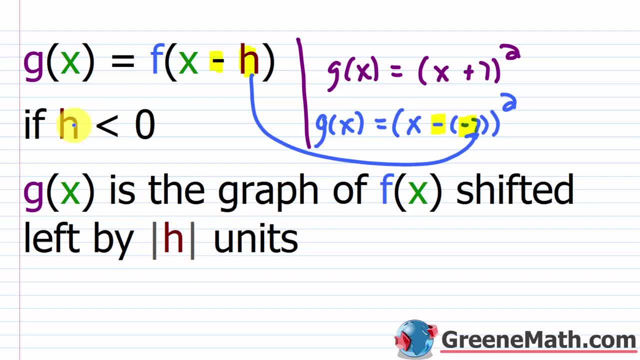 by the absolute value of h units. Again, because h here is less than zero, h is negative, So the absolute value of negative seven is seven. So it would shift to the left by seven units. But I don't recommend doing this. 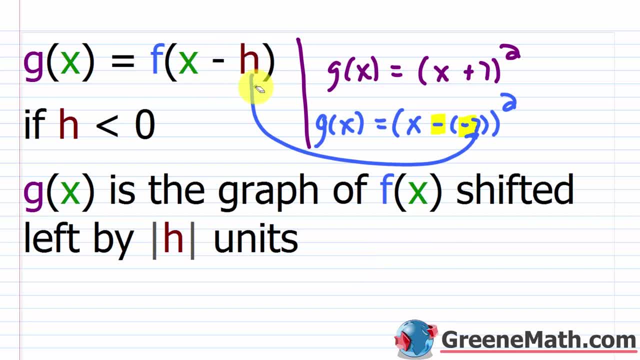 This is something you can do when you first start. The way I want you to think about this is: what do I need to do to undo what's being done to x? In this case, we're adding seven. We're adding seven to x. 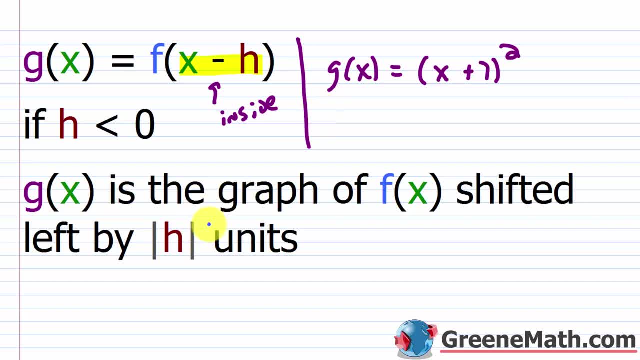 plus a positive. so you got to be thinking this way, that to write it like this and follow this rule, i would say g of x is equal to the quantity x minus a negative seven and that amount squared. so following this, let me just kind of erase this real quick. following this, i've got my minus and 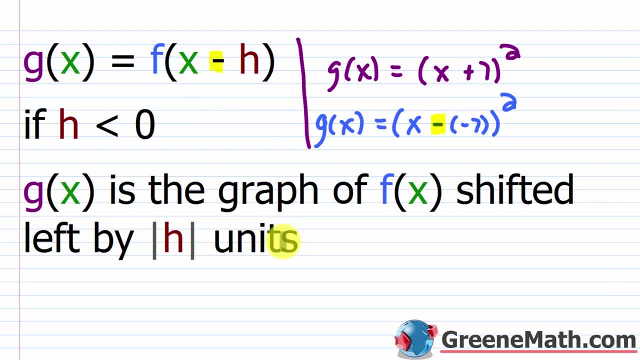 i've got my minus so i've written it perfectly in line with the formula they've given me. so i know that h now is going to be negative seven. okay, h is negative seven. so just following the rule g of x, is the graph of f of x shifted left by the absolute value of h units again, because h here is less than. 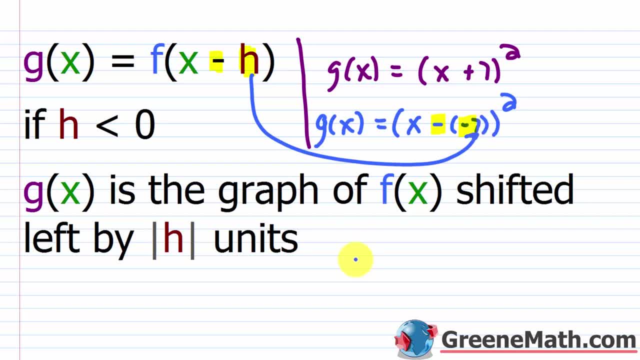 zero h is negative, so the absolute value of negative seven is seven. so it would shift to the left by seven units. but i don't recommend doing this. this is something you can do when you first start. the way i want you to think about this is: what do i need to do to undo what's being? 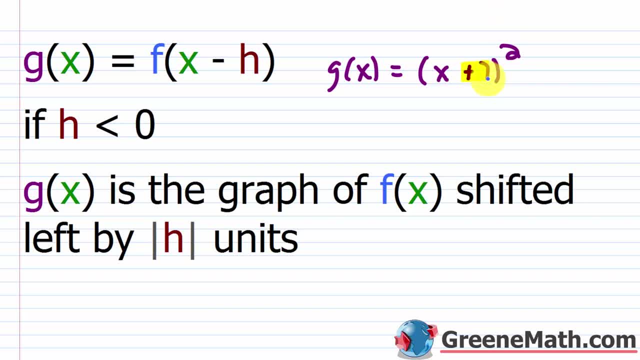 done to x. in this case, we're adding seven. okay, we're adding seven to x. to undo that, i need to subtract seven. okay, i need to subtract seven. and if i think about that, okay, for the same y value, now x needs to be seven units less. okay, if i think about that, on the horizontal axis, i would go seven units to the left. 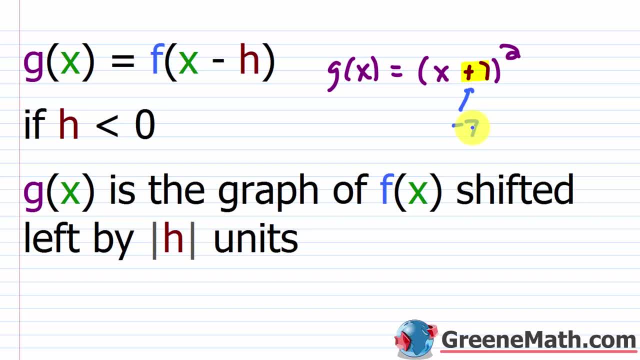 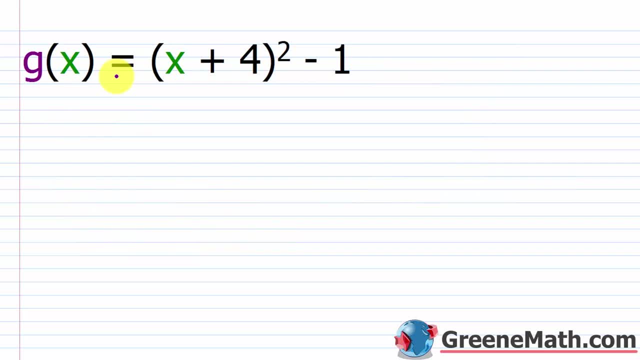 right, that's how i decrease on the x axis. so just figure out what you need to do to undo what's being done to x and then consider your shift that way. so let's just look at some examples real quick. we have: g of x is equal to the quantity x plus four squared and then minus one, so our parent function. 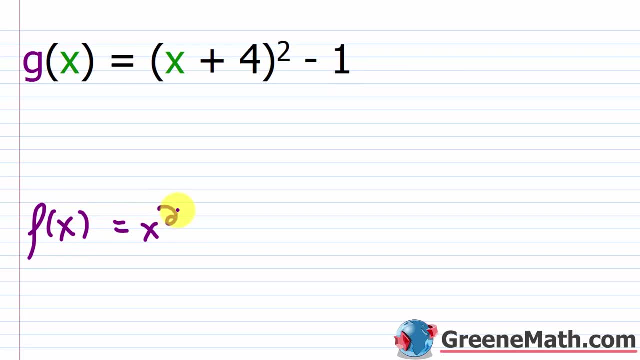 here would be: f of x is equal to x squared, and what you'll notice is that this part right here is happening inside the function. right, i could plug in an x plus four, kind of in for x, in f of x and i could obtain that part. then i have this minus one. this is happening outside the function. 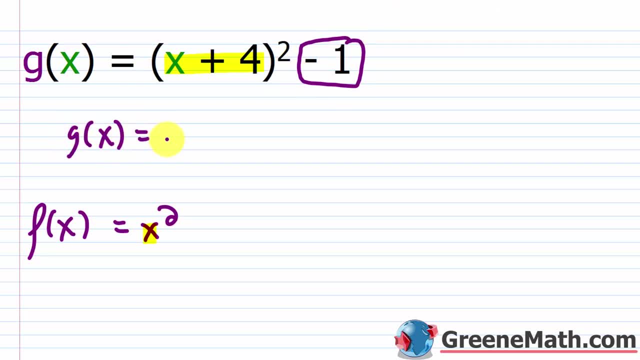 if i wanted to think about this, i could say that g of x is f of x plus four and then minus one, right? that would be the notation if you wanted to describe it. but essentially, once we have that down right, we don't need to write that each time, we just think. 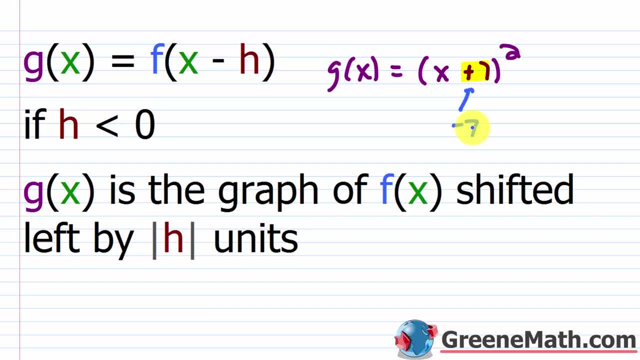 To undo that I need to subtract seven. I need to subtract seven And if I think about that, for the same y value now x needs to be seven units less. If I think about that on the horizontal axis, I would go seven units to the left. 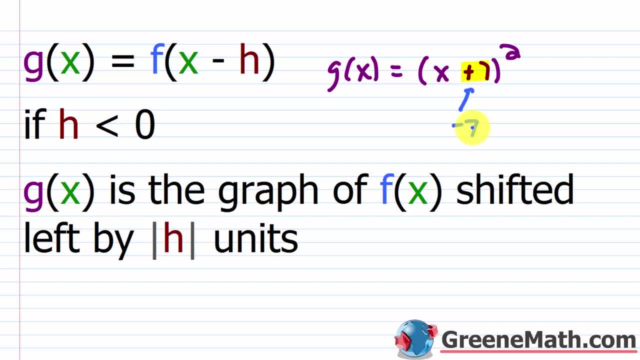 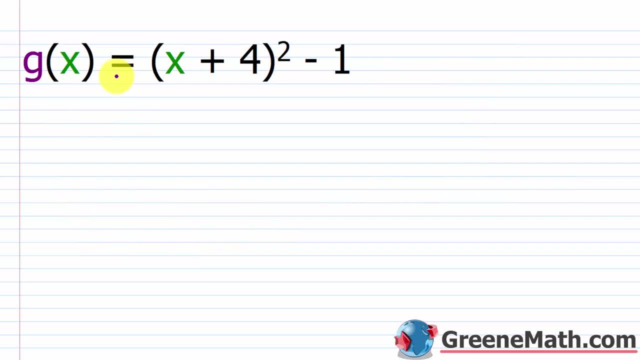 That's how I decrease on the x axis. So just figure out what you need to do to undo what's being done to x and then consider your shift that way. So let's just look at some examples real quick. We have g of x is equal to. 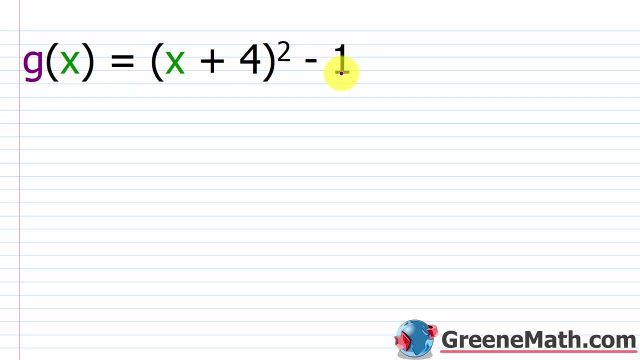 the quantity x plus four squared and then minus one. So our parent function here would be: f of x is equal to x squared, And what you'll notice is that this part right here is happening inside the function. I could plug in an x plus four. 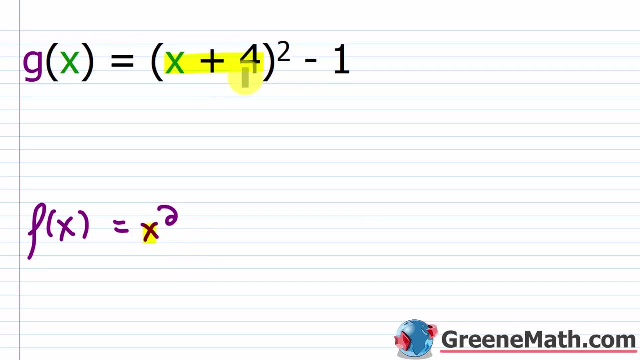 kind of in for x, in f of x, and I could obtain that part. Then I have this minus one. This is happening outside the function. If I wanted to think about this, I could say that g of x is f of x plus four. 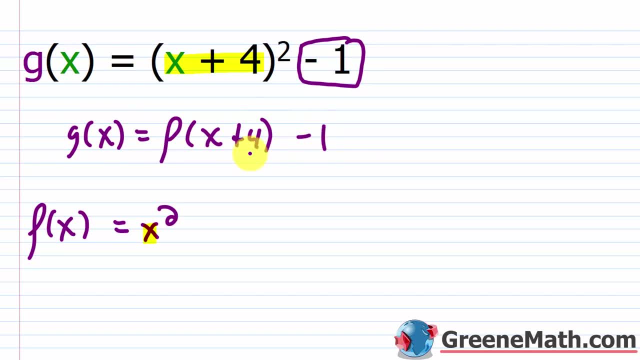 and then minus one. That would be the notation if you wanted to describe it. But essentially, once we have that down, we don't need to write that each time. We just think about what's going on. So this part's just inside the function. 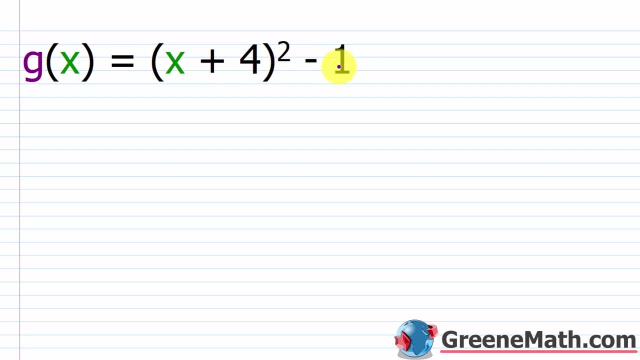 This part's outside. Now, if you want to use those rules that I gave you earlier, feel free. You can do that when you first start. But the quickest way when you're looking at this stuff is just to think about for the inside of the function part. 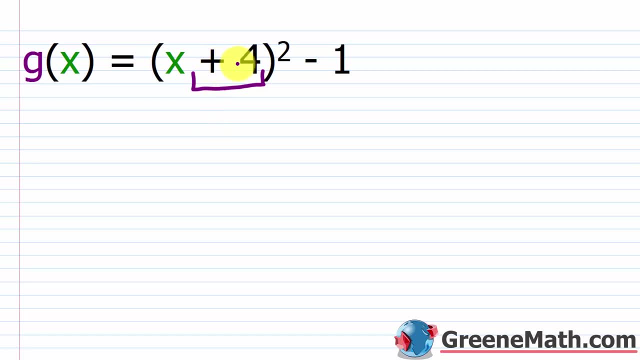 what's going to undo what's being done to x? I have a plus four there, So to undo that I need to subtract four away. So if I'm subtracting four away, what that's telling me is that for a given y value, 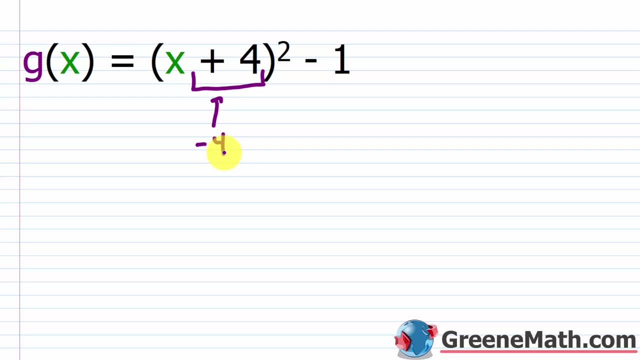 x now needs to be four units less, So that's going to shift the graph left by four units. So I can say that we're going to shift, or we'll really just say shifts left by four units, And again this is kind of counterintuitive. 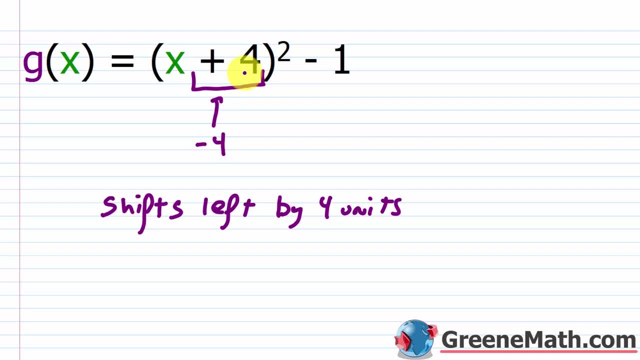 You see this, x plus four. You're thinking, oh, I'm shifting to the right by four units, But it ends up being that you're shifting to the left by four units. Now, additionally, you have this minus one that happens outside the function. 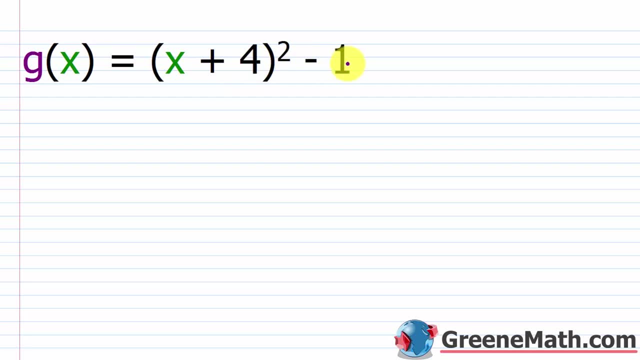 about what's going on. so this part's just inside the function, this part's outside. now, if you want to use those rules that i gave you earlier, feel free. you can do that when you first start. but the quickest way when you're looking at this stuff is just to think about: okay for the inside of the. 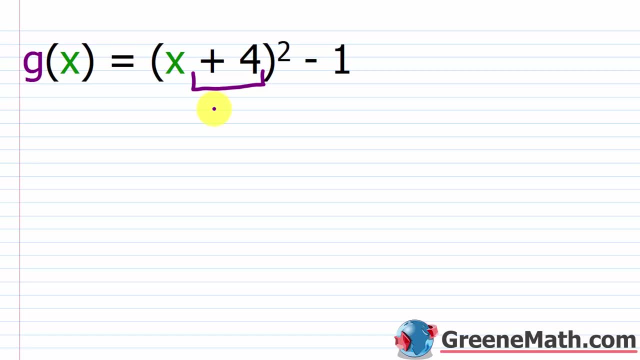 function part. what's going to undo what's being done to x? i have a plus four there, so to undo that i need to subtract four away. okay, so if i'm subtracting four away, what that's telling me is that for a given y value, x now needs to be four units less, so that's going to shift the graph left. 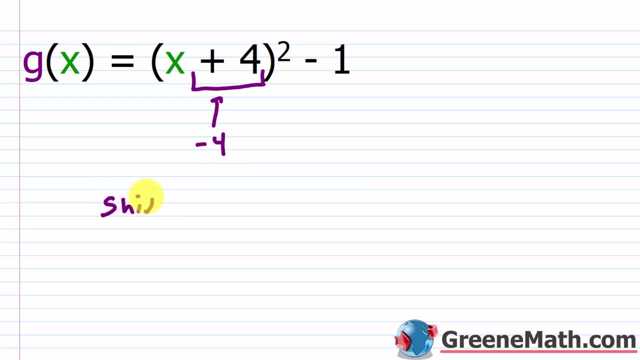 by four units, so i can say that we're going to shift, or we really just say shifts left by four units. okay, and again, this is kind of counterintuitive, right, you see this, x plus four. you're thinking, oh, i'm shifting to the right by four units, but what you're going to do is you're. 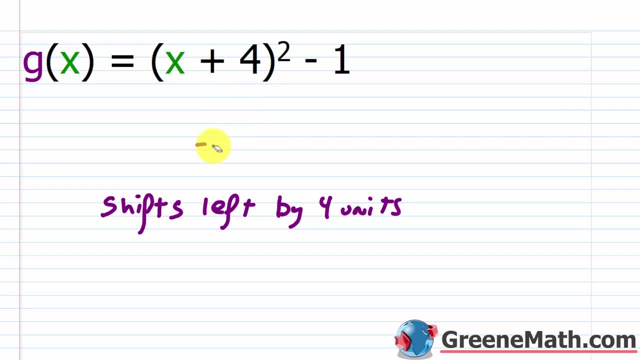 going to shift to the left by four units. now, additionally, you have this minus one that happens outside the function. this one's very straightforward, right. if i'm subtracting away one, then i'm just shifting down by one unit. if this was something like plus one, i would just shift. 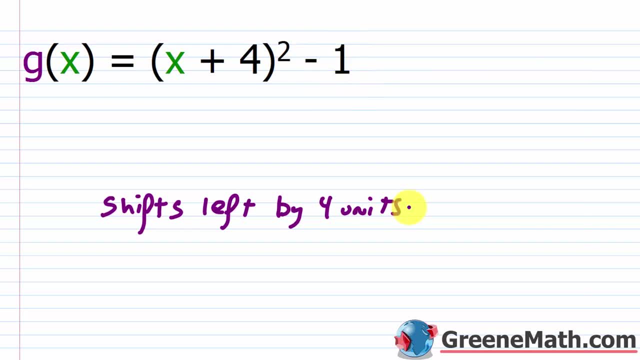 up by one unit, okay, but it's minus one in this case. so, additionally, we're also going to say it shifts down by one unit, okay. so those are the two things that are going to occur. so, based on that original graph, f of x equals x squared, we would shift every point to the left. 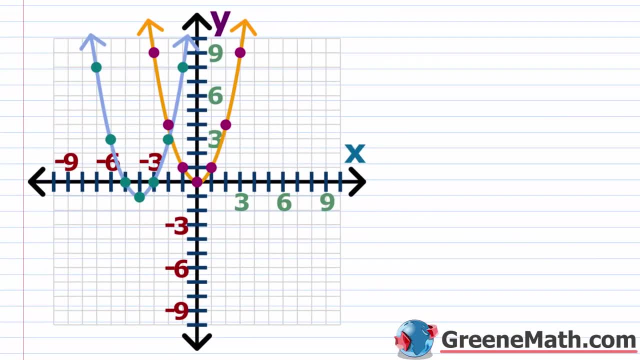 by four units and down by one unit. so graphically we can see this: our orange graph is f of x equals x squared. our blue graph, our light blue graph, is g of x equals the quantity x plus four squared minus one. so to kind of graph the blue one. quickly. just take these points that you already know and 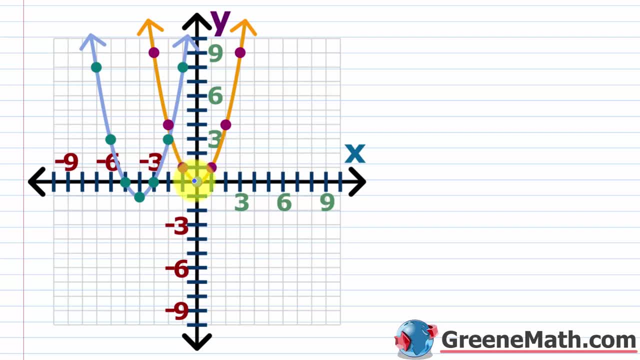 love like zero, comma zero. shifted: four units left and one unit down. so one, two, three, four, one unit down, right, you can do as many of these as you need to. so let's say i take this point, i'm going to go one, two, three, four, one unit down. okay, so on and so forth. that's how you. 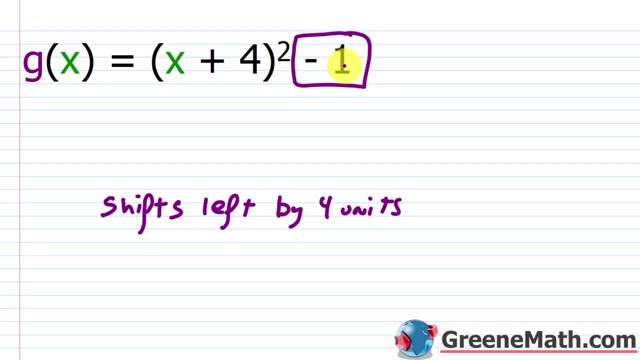 This one's very straightforward: If I'm subtracting away one, then I'm just shifting down by one unit. If this was something like plus one, I would just shift up by one unit, But it's minus one in this case. So additionally we're also going to say it shifts. 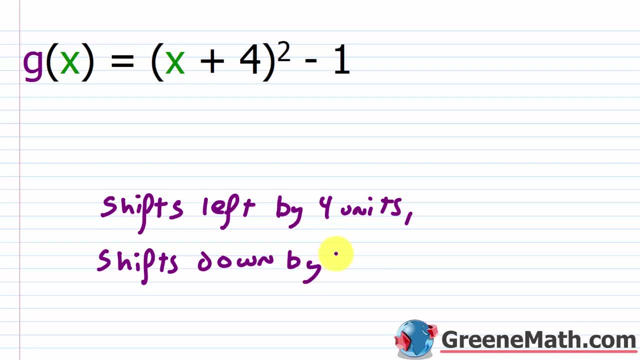 Down by one unit. Okay, so those are the two things that are going to occur. So, based on that original graph, f of x equals x squared, we would shift every point to the left by four units and down by one unit. So graphically we can see this: 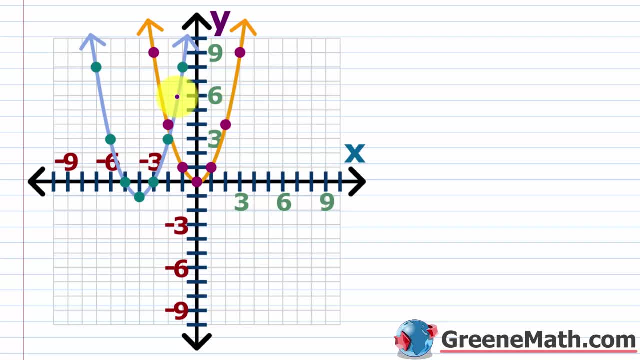 Our orange graph is f of x equals x squared. Our blue graph, our light blue graph, is g of x equals the quantity x plus four squared minus one. So to kind of graph the blue one. quickly just take these points that you already know and love. 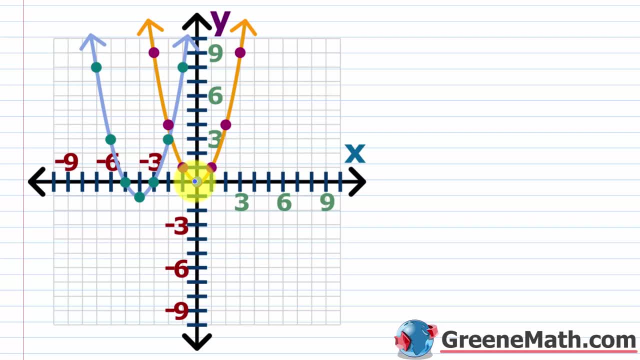 like zero comma zero, shifted: four units left and one unit down. So one, two, three, four, one unit down, Right, you can do as many of these as you need to. So let's say I take this point, I'm going to go one, two, three, four, one unit down. 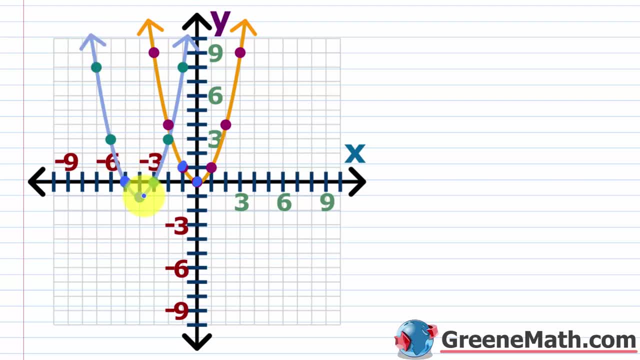 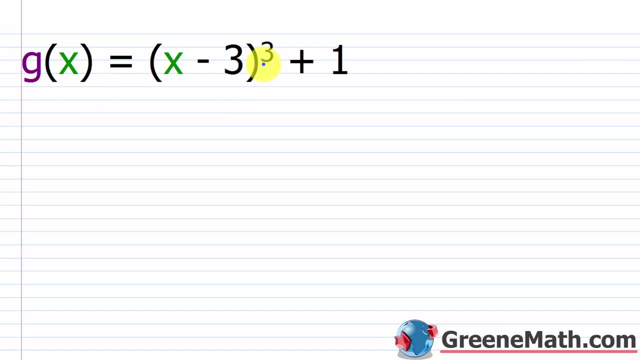 Okay, so on and so forth. That's how you could quickly sketch your graph. All right, let's take a look at another one. So now we have: g of x is equal to the quantity x minus three cubed and then plus one. 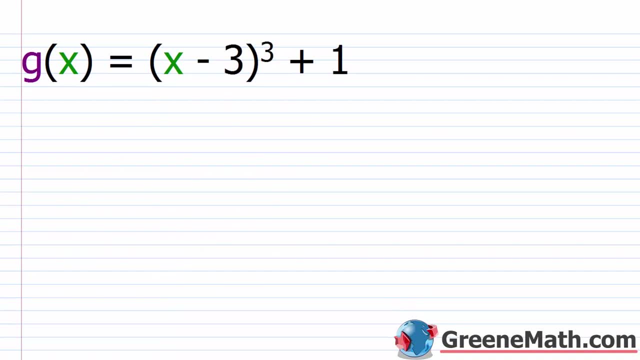 could quickly sketch your graph. all right, let's take a look at another one. so now we have: g of x is equal to the quantity x minus three cubed and then plus one. so this guy is based on f of x equals x cubed. right, that would be your parent function. so this part right. here is the inside, the 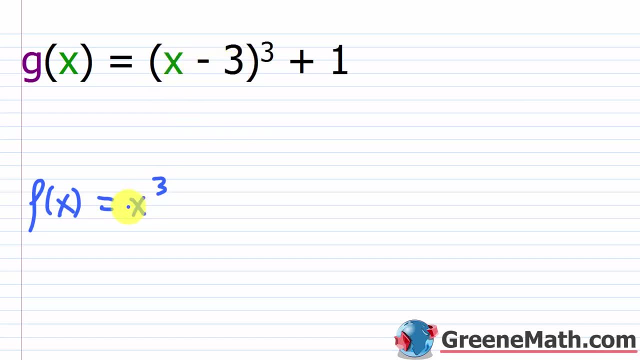 function part right. i could plug in an x minus three kind of in for x in this original function. so if i had f of x minus three i would have the quantity x minus three cubed okay. so that would give you this part kind of right here. and then i have that plus one that happens outside of the 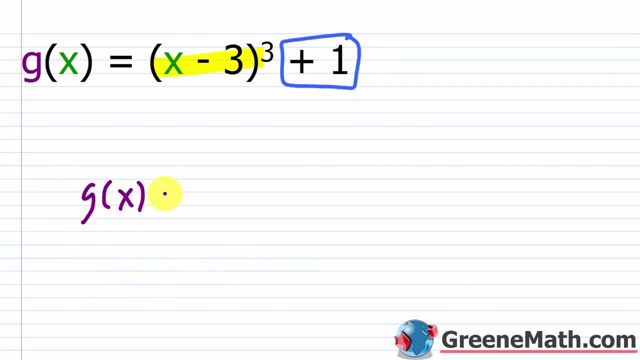 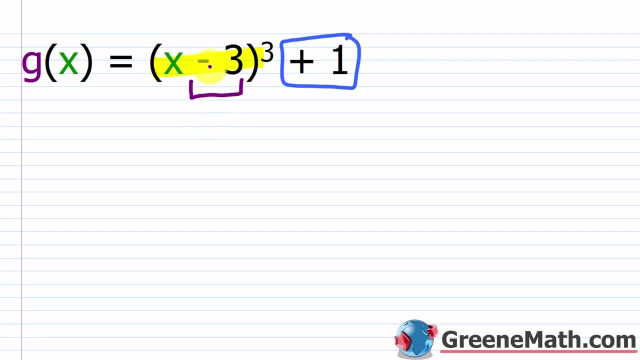 function part. i think about what i need to do to undo what's being done to x. in this case i'm subtracting three away from x, so to undo that i would add three. right, so if i add three, then for a given y value, x now needs to be three units larger, okay, so again, i'm adding three, so that 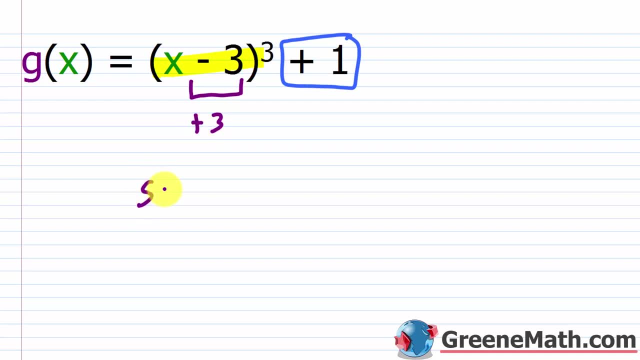 means i'm shifting to the right by three units, so this shifts right by three units. okay, now this plus one here again, that's outside the function. it's just telling me we're shifting up by one unit. so we're just going to say shifts up by one unit. all right, so graphically again. 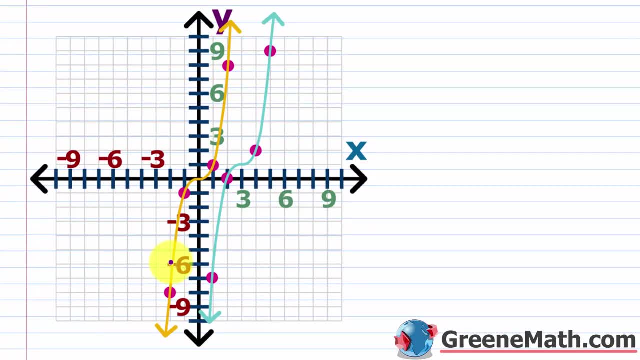 our graph in orange is our original f of x equals x cubed. and then this guy right here in light blue is my g of x equals x minus three, that quantity cubed and then plus one. so every given point. let's just take this one for example. 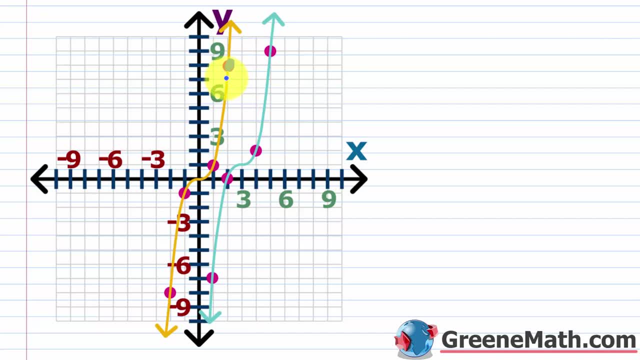 here let's use our calculator to see what we're getting. so we're going to shift to the right by three units and it's going to shift up by one unit. so this would go one, two, three units to the right, one unit up. you could take this point right here: you can go one, two, three years to the right one. 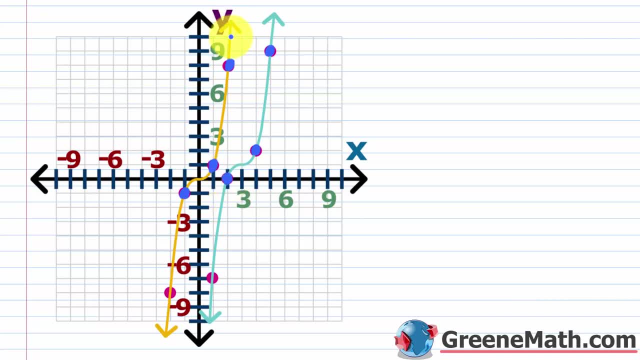 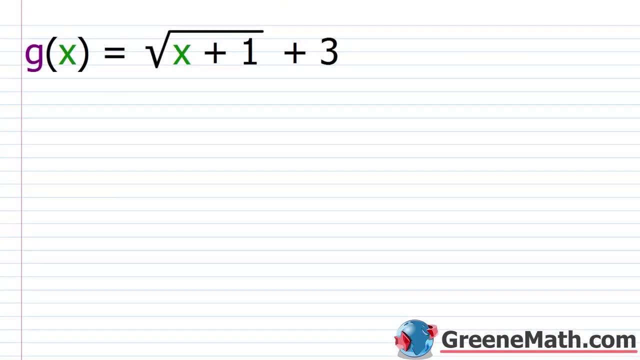 unit up this guy right here, one, two, three years to the right. one unit up right, so on and so forth. if you already know the graph of kind of f of x equals x cubed, then it's easy to graph this kind of g of x graph. all right, let's take a look at another one. 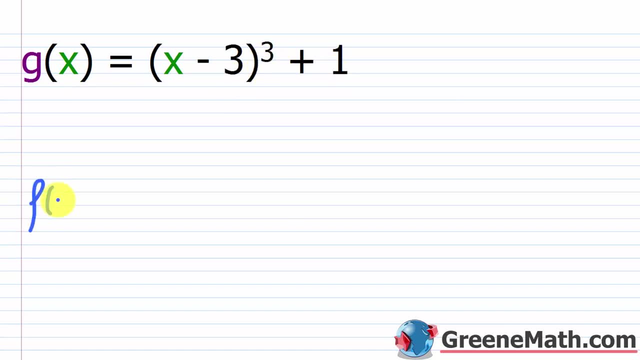 So this guy is based on f of x equals x cubed, Right, that would be your parent function. So this part right here is the inside, the function part. Right, I could plug in an x minus three kind of in for x in this original function. 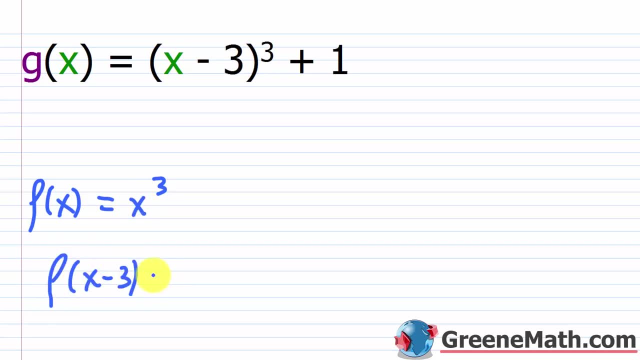 So if I had f of x minus three, I would have the quantity x minus three cubed. Okay, so that would give you this part kind of right here. And then I have that plus one That happens outside of the function, right. 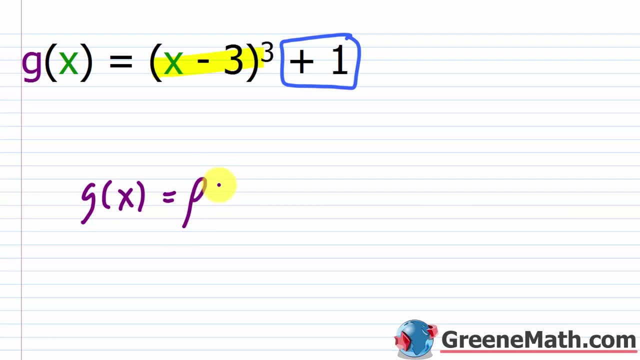 So really, we could say that g of x is equal to f of x minus three, and then plus one, Right? if you wanted to define it that way, All right. so what's going on here? is that, again from the inside, the function part. 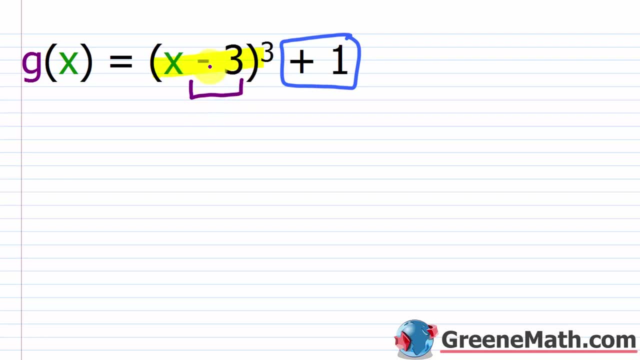 I think about what I need to do to undo what's being done to x. In this case I'm subtracting three away from x, So to undo that I would add three, Right? so if I add three, then for a given y value. 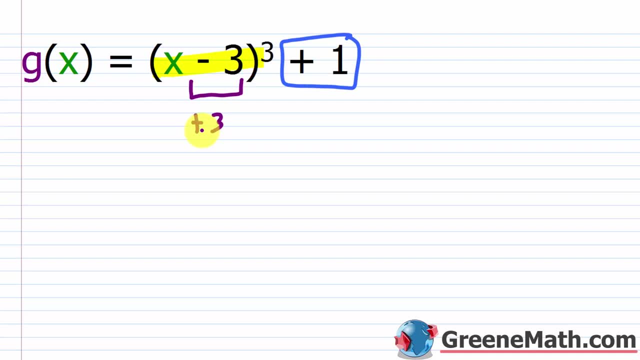 x now needs to be three units larger, Okay. so again I'm adding three. So that means I'm shifting to the right by three units. So this shifts right by three units. Okay, now this plus one here. again, that's outside the function. 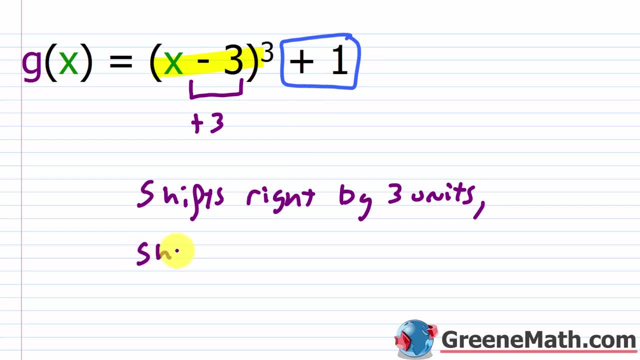 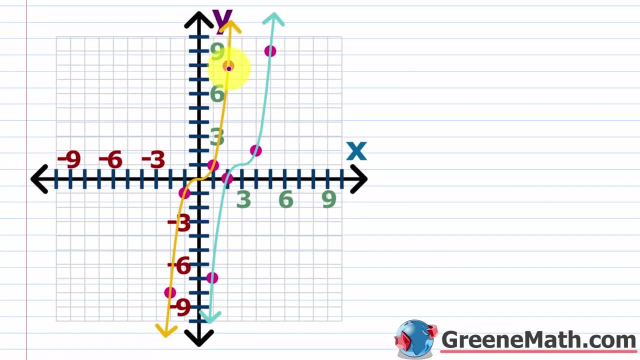 It's just telling me we're shifting up by one unit. So we're just going to say: shifts up by one unit, All right. so graphically again, our graph in orange is our original f of x equals x cubed. And then this guy right here: 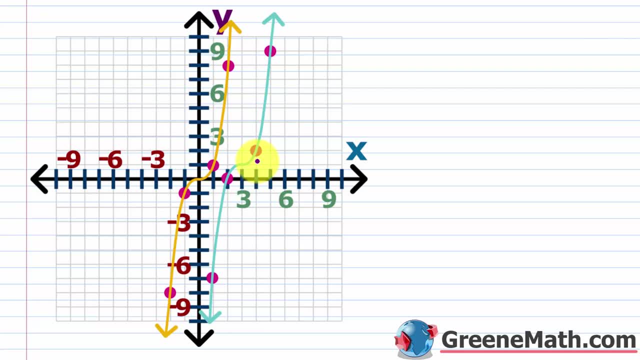 in light blue is my g of x equals x minus three, that quantity cubed and then plus one. So every given point- let's just take this one, for example- is going to shift to the right by three units and it's going to shift up by one unit. 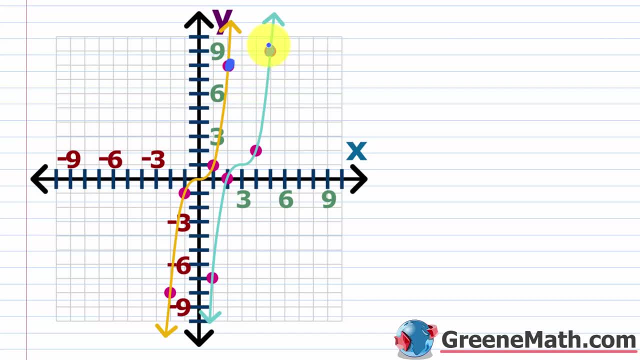 So this would go one, two, three units to the right, one unit up. You could take this point right here. you could go one, two, three units to the right, one unit up, This guy right here. one, two, three units to the right. 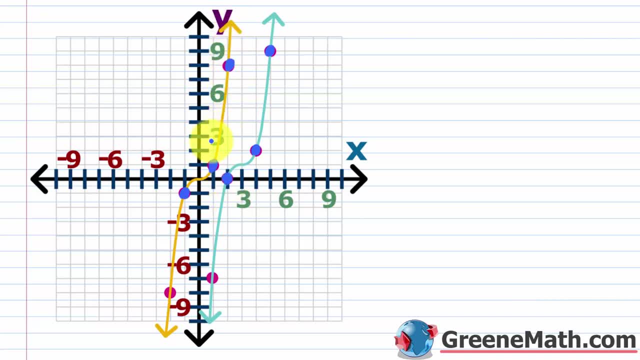 one unit up Right, so on and so forth. If you already know the graph of kind of f of x equals x cubed, then it's easy to graph this kind of g of x graph. All right, let's take a look at. 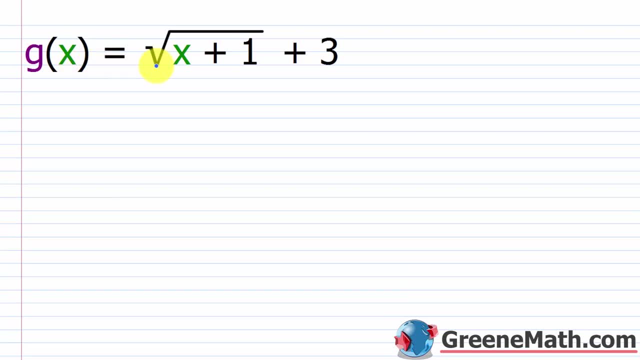 another one. So suppose we have: g of x equals the square root of x plus one and then plus three. So this part right here is what's going on on kind of the inside, This part right here is the outside. Okay, so in other words, let me just write: 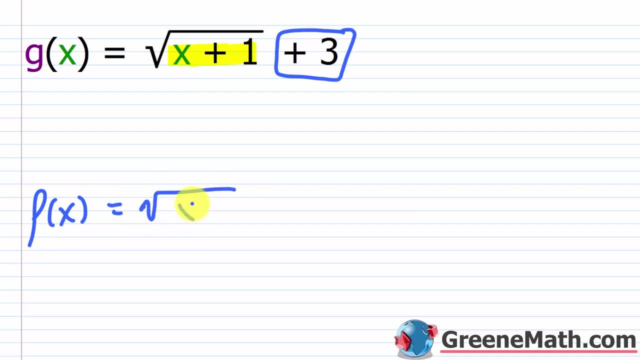 this one more time. So f of x equals the square root of x. If I plugged in an x plus one for x in this function, again that's what's happening on the inside of the function. Can I replace x with that? 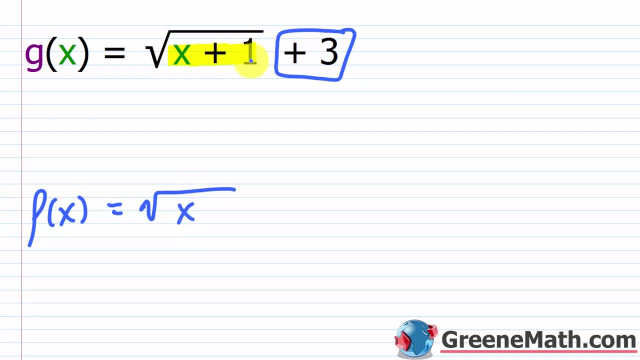 So in this case, can I replace x with the quantity x plus one? Well, yeah, that's how I get that. Okay, so now we need to think about, for the inside part, how can I undo what's being done to x? Well, I have this plus. 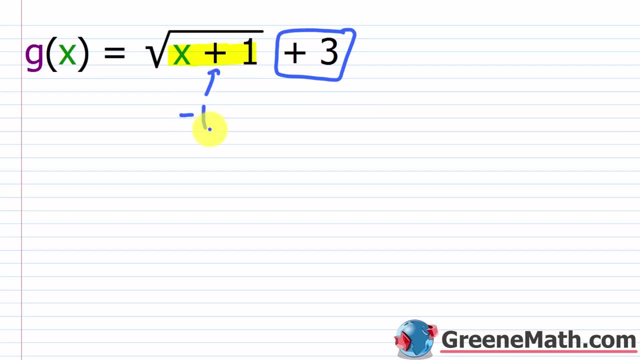 one. okay, I'm adding one, so I need to subtract one away to undo that. So again, for a given y value, x needs to be one unit less. So I would just say we're going to shift left, We'll say shifts left. 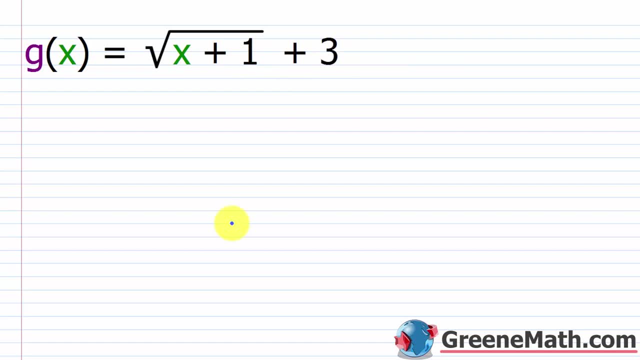 the square root of x plus 1 and then plus 3.. So this part right here is what's going on on, kind of the inside. This part right here is the outside. Okay, So in other words, let me just write this one more time: So f of x equals the square root of x. If I plugged in an x plus 1. 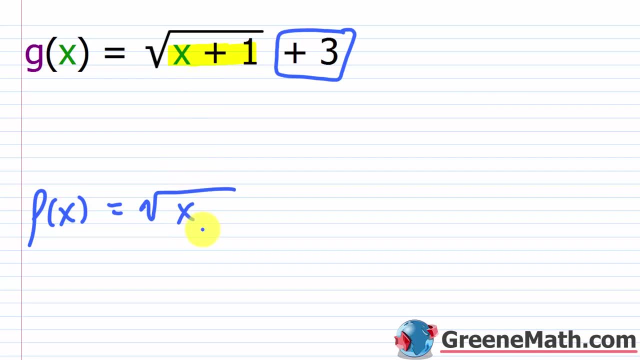 for x in this function. again, that's what's happening on the inside of the function. Can I replace x with that? So in this case, can I replace x with the quantity x plus 1?? Well, yeah, that's how I get that. Okay, So now we need to think about for the inside part. 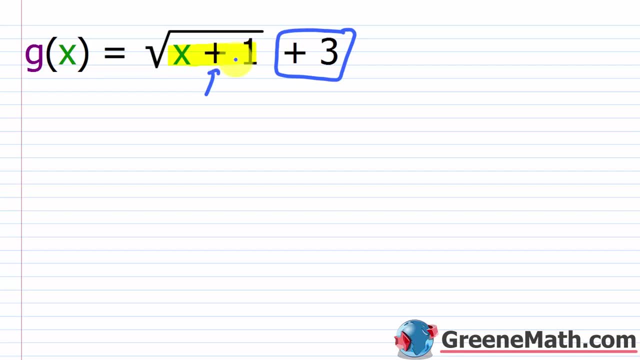 how can I undo what's being done to x? Well, I have this plus 1.. Okay, I'm adding 1.. So I need to subtract 1 away to undo that. So again, for a given y value, x needs to be one unit less. 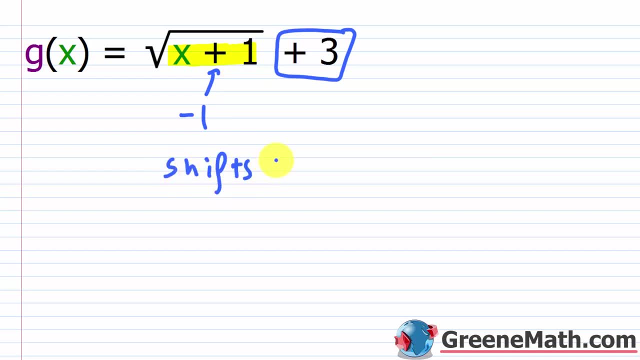 So I would just say we're going to shift left. We'll say shifts left by one unit, And then this plus 3 on the outside of the function. that just tells me we shift left. So we're going to shift left by one unit, And then this plus 3 on the outside of the function. 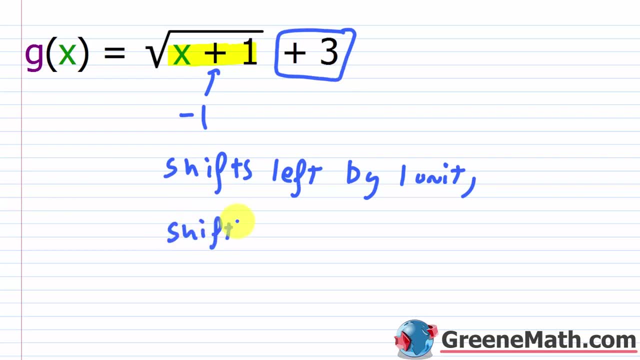 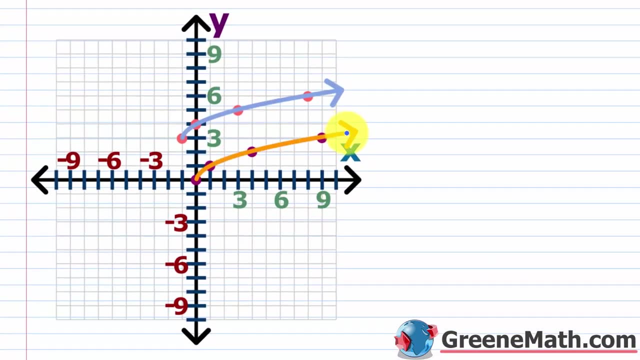 that just tells me, we shift left by one unit, And then this plus 3 on the outside of the function up by three units, And then we'll say: shifts up by three units. So graphically the orange graph is f of x, equals the square root of x. And then the light blue graph is g of x, is the square root. 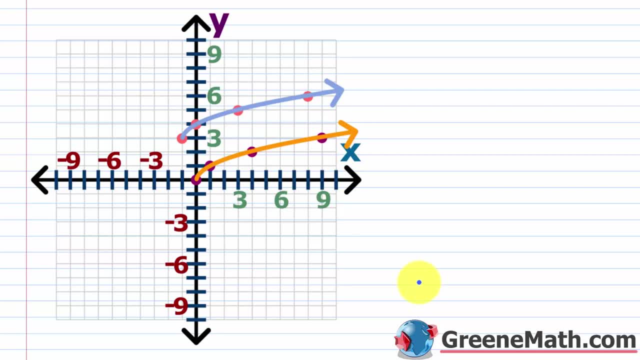 of x plus 1.. And then you have plus 3 on the outside. So again, every given point is going to be shifted one unit to the left and three units up. So let's just take this point. 0,0 on the. 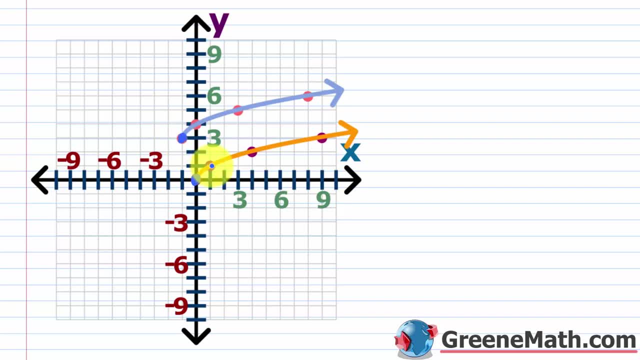 outside: 1,, 2,, 3, and then one unit to the left, Right, so on and so forth. So this point up: 1,, 2,, 3,, one unit to the left. So again, if you know this graph and you should memorize. 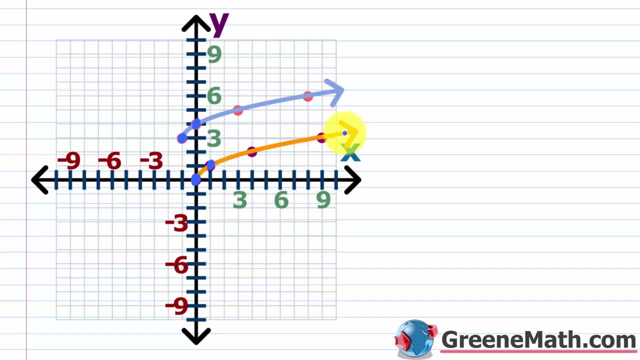 the graph of f of x equals the square root of x, then you can quickly graph this kind of g of x. Once you figure out what the shifts are, you can graph this guy, if you need to, real quickly and then shift the point and then sketch your graph. 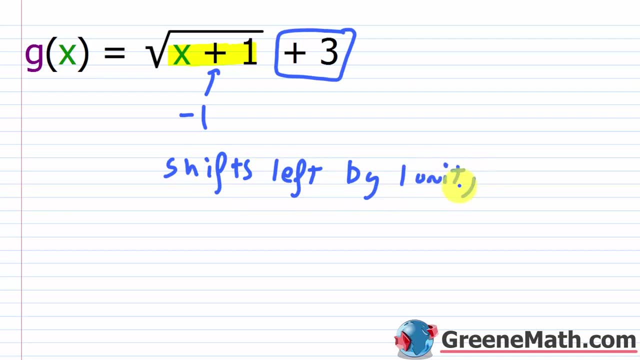 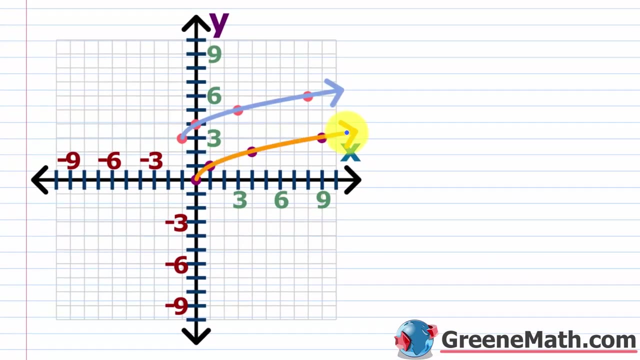 By one unit And then this plus three. on the outside of the function, that just tells me we shift up by three units. And then we'll say: shifts up by three units. So graphically the orange graph is: f of x equals the square root of x, and then 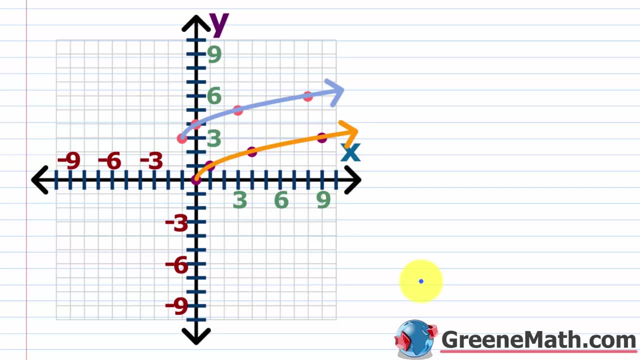 the light blue graph is g of x, is the square root of x plus one, and then you have plus three on the outside. So again, every given point is going to be shifted one unit to the left and three units up. So let's just take this point: zero, comma zero. 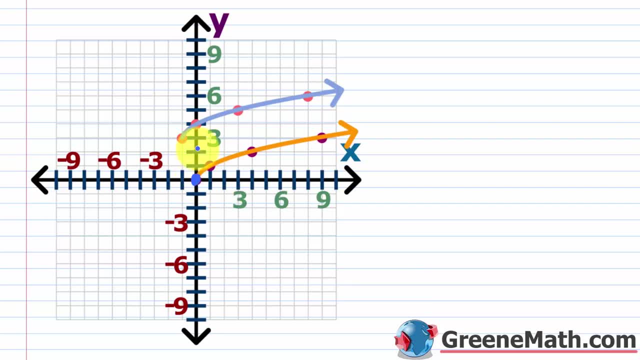 on the original. It goes up one, two, three and then one unit to the left, Right, so on and so forth. So this point up: one, two, three, one unit to the left. So again, if you know this graph, 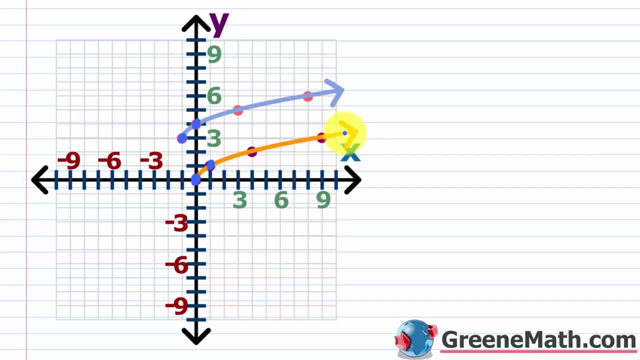 and you should memorize the graph of f of x equals the square root of x. then you can quickly graph this kind of g of x. once you figure out kind of what the shifts are, You can graph this guy if you need to real quickly and then 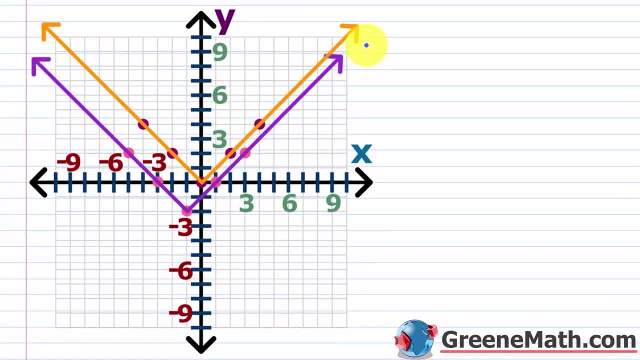 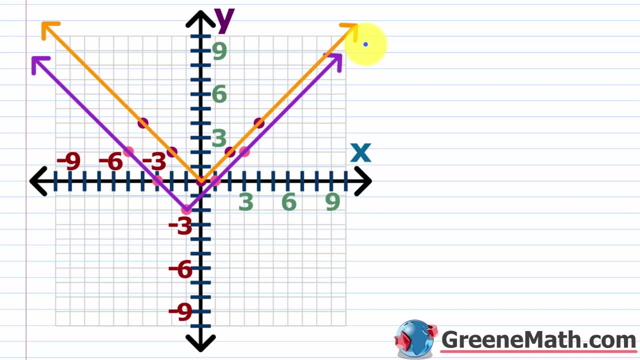 shift the point and then sketch your graph of the other one. So for the last example, we want to look at this kind of purple graph and we want to determine kind of the function. So the orange graph is kind of a reference. It's our. 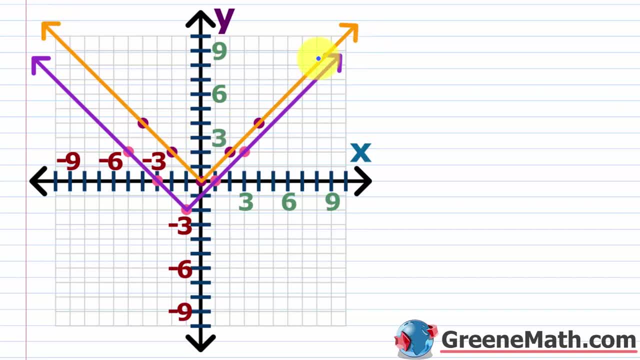 kind of parent function. So you should recognize this at this point. It has this v shape. that's a very signature graph. It's: f of x is equal to the absolute value of x, right? So this purple graph, again, the parent function will be f of x. 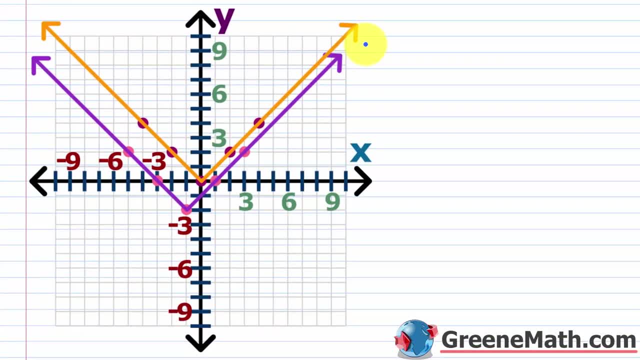 of the other one. So for the last example, we want to look at this purple graph, we want to determine the function. So the orange graph is kind of a reference. It's our kind of parent function. So you should recognize this at this point. 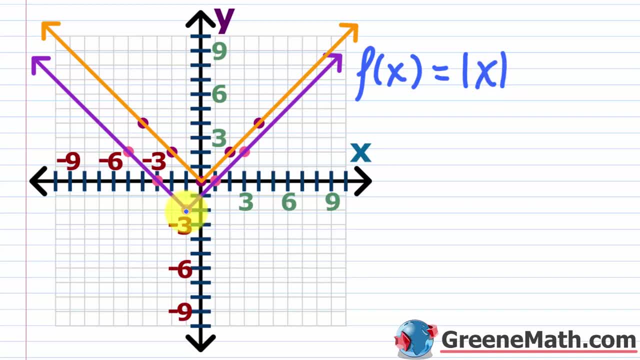 equals the absolute value of x. How can we define this graph of this purple function? Let's call it g of x and let's just look at what happens. You just look at the points. We know this is the lowest point here and that gets transferred to. 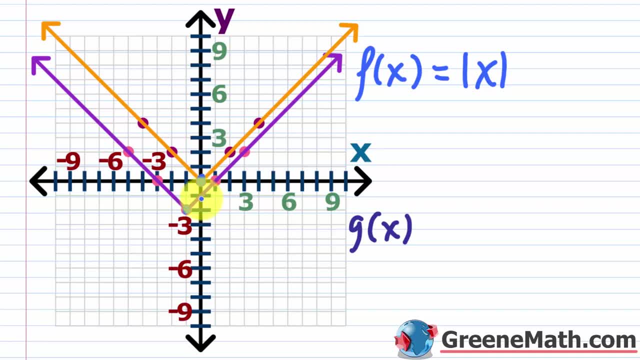 there. So I would go what? I would go down one, two and to the left one. So we went down by two and we went left by one. Okay, So let's see if we can figure that out. So down by two means I subtract away. 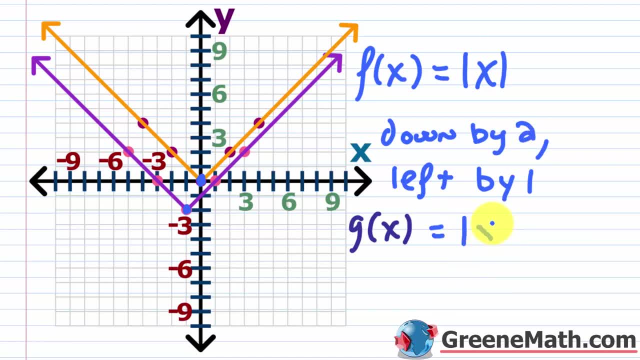 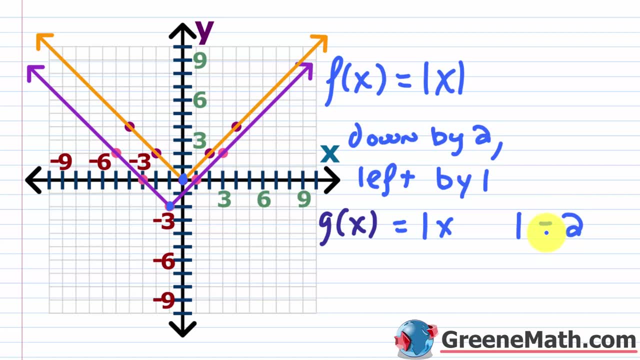 two on the outside of the function. So let's say we have the absolute value of x and I'll just leave some space Again. if I go down by two, I have minus two outside the function. Or you can put plus negative two if you want to, It doesn't.